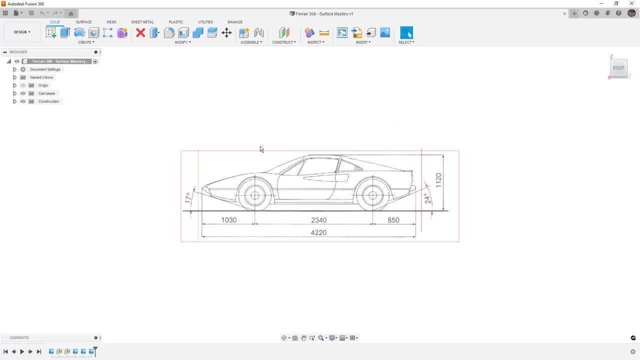 to do is we're going to use this as our basis to create curves in 3D. Now you can go to the description of the video and download the data set which has these blueprints set up for you. What we're going to do is get started by first creating a sketch on the side. 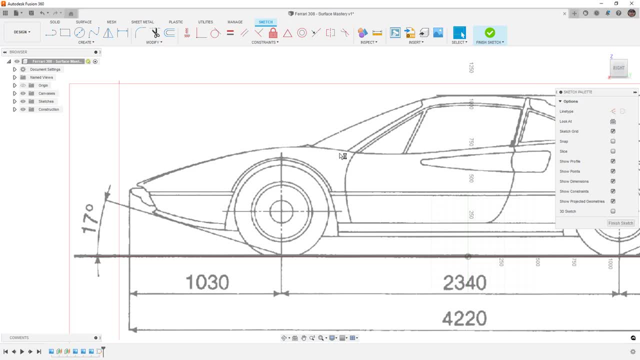 and we're going to look at the shape of the fender from the side. Now, this is an important consideration because there's a couple design decisions that we have to make at this stage When we're creating curves in 3D. the most efficient way that I found is to 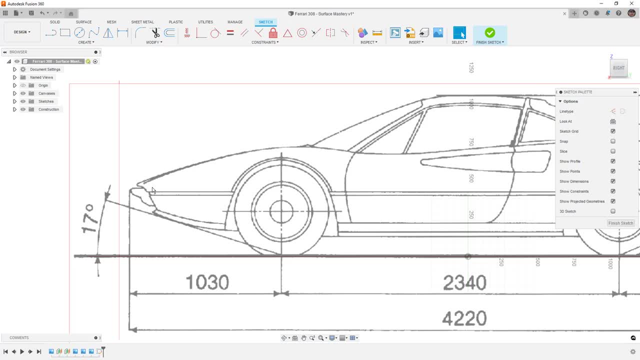 project 2D curves out until they intersect in 3D. This means that we need to be extremely mindful of the start and end of those curves and the direction in which we're modeling them. For something like a front fender, we have a good view from the side and we have a good view from the. 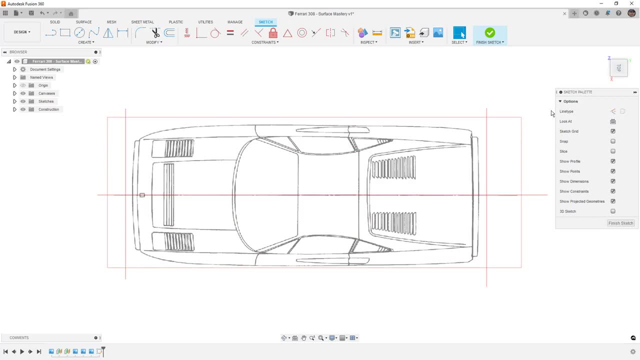 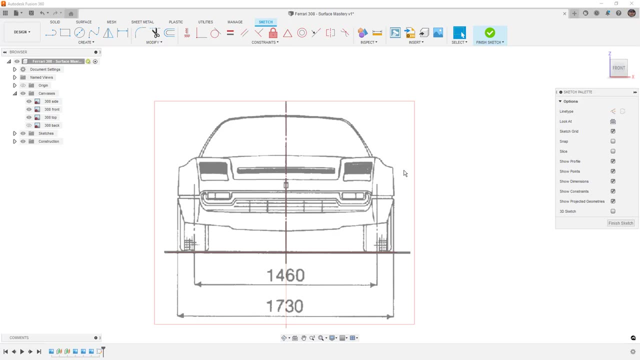 top, We can see all the geometry that we need to see here. However, if we look at the design from the front, you can see that we are going to be missing a portion of it- I'm going to hide the back for now, so it's not obscured- And what we see here is that 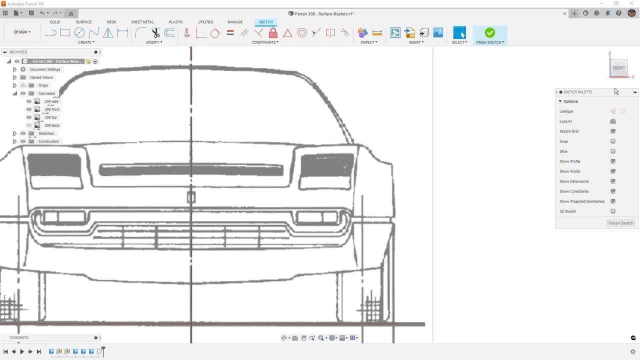 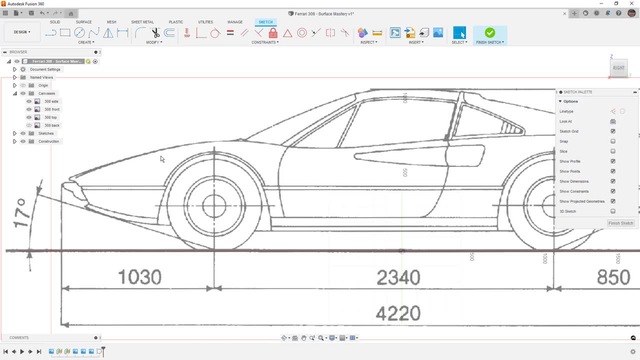 we can only see to the crest or the top position above the wheel When we look at it from the side. as soon as that curve starts to taper back down, we can no longer see that geometry from the front. So this is important, because this means that we really need to think about the direction of our 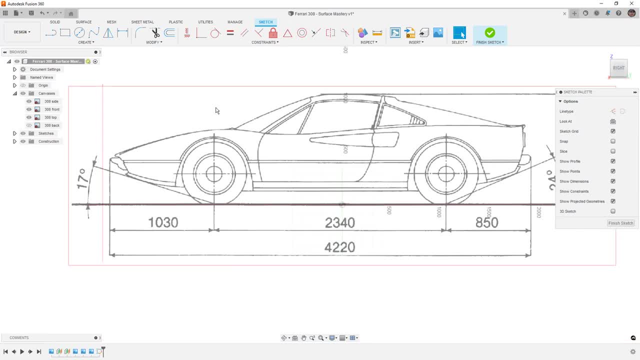 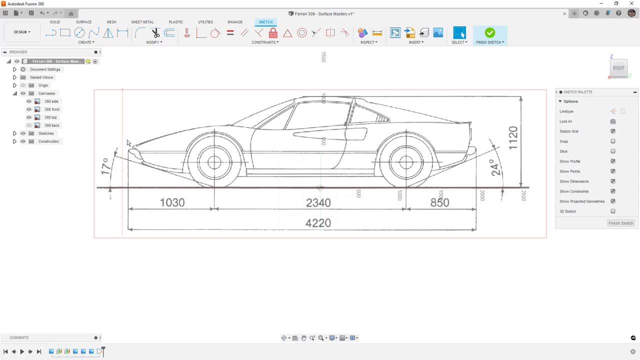 sketches. So for us we're going to go from the side and the top. Then we need to think about how much of the curve we're drawing With surfaces. it's often easier for us to overbuild the surfaces and trim them back. It's going to be a much cleaner approach. 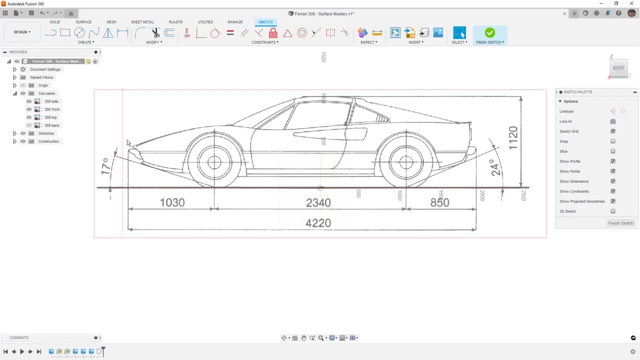 than if we make them too small and we have to extend them. So keep in mind that we can always go back and we can trim these surfaces, But when you're building a model like this, you generally aren't hoping for it to be able to update very easily. So we're going to get started with a 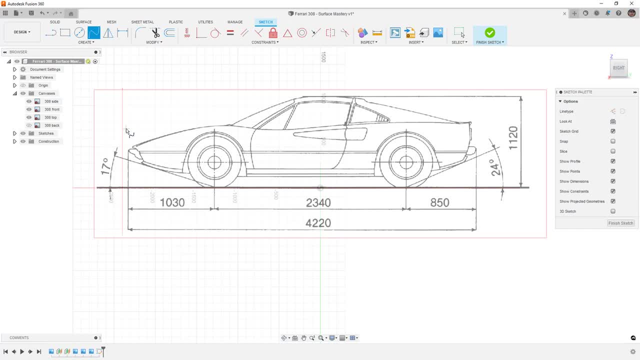 spline and I'm going to be using FitPoint splines for this example, simply because the control points will be directly on the curve, So we're going to go from the side and the top position above the wheel. That means it's a little bit easier for us to visualize these when we're looking at a blueprint. 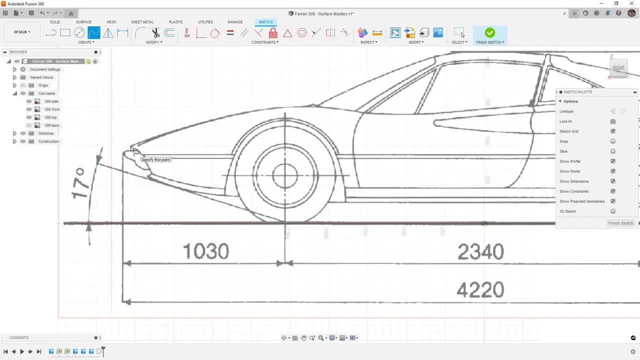 So I'm going to start ahead of the front here Now keep in mind that again the fender sort of rolls here and we're going to move this back in just a second And I'm going to do two curves here. I'm going to do one curve that just goes to the base of the A-pillar, and then we're going to 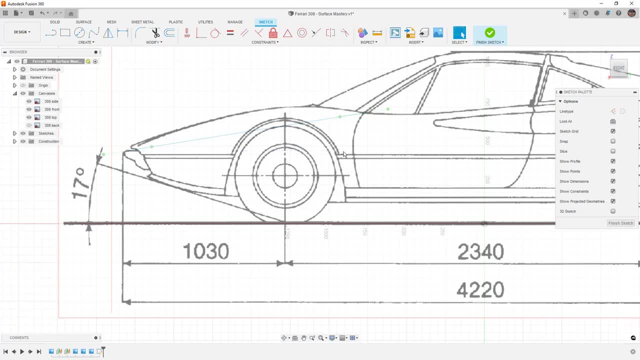 come back and we're going to take a look at doing the entire side. So I'm going to hit escape to get off my spline tool and I'm going to begin manipulating these handles. You can see, just by moving the rear handle I'm going to be able to manipulate these handles. So I'm going to. 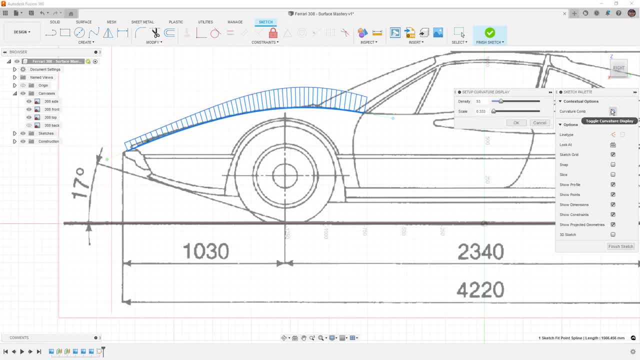 get pretty close. I'm going to select the spline and turn on my curvature combs. I've got my density set to about 50, and the scale you can see here is 0.33.. You can increase or decrease these It. 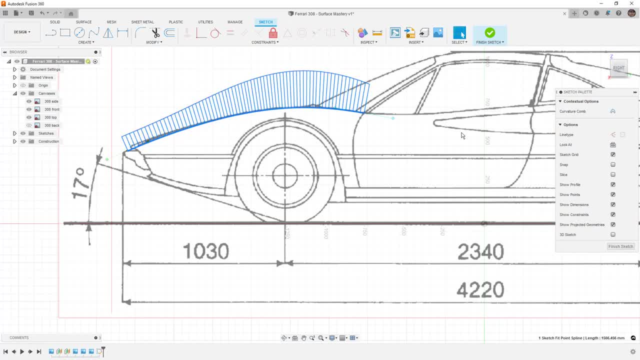 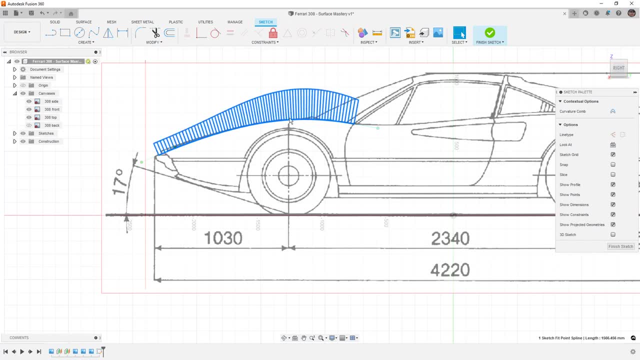 doesn't really matter, but sometimes increasing the density can visually help. So when we're looking at this, what I want to see is any areas where we're expecting a large change in curvature, So for example, the top of the fender. here we would want to see a bit of a longer line on the. 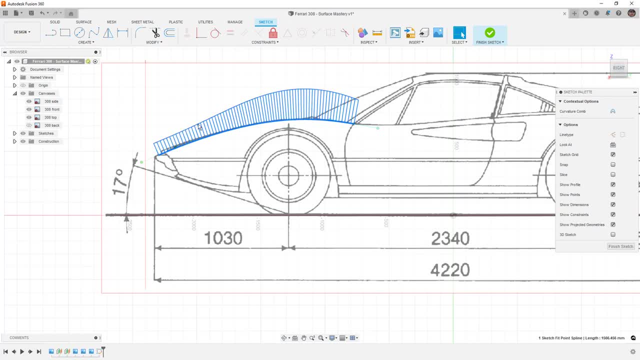 curvature comb and anywhere that it starts to change, we're going to want to see a bit of a consistent curve. What we don't want to see is going to be a drastic change in curvature or an inflection point. This means that we're going from convex to concave here. So I'm going to do: 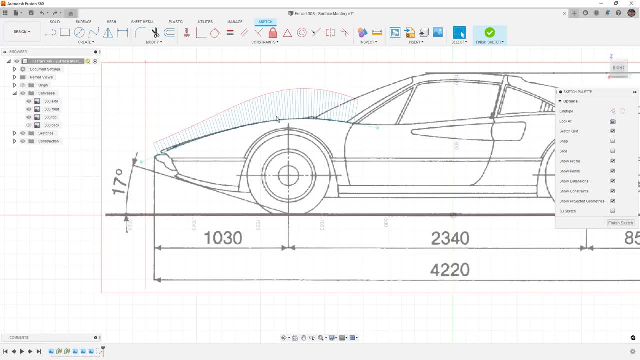 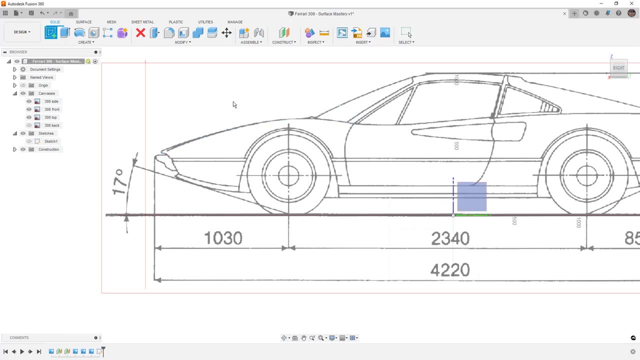 control Z to undo and I like the way that that curve looks, So I am going to be happy with that. I'm going to finish the sketch. I'm going to hide the sketch temporarily because I want to show the same process, overbuilding it for the entire car and how this is a potentially more complicated 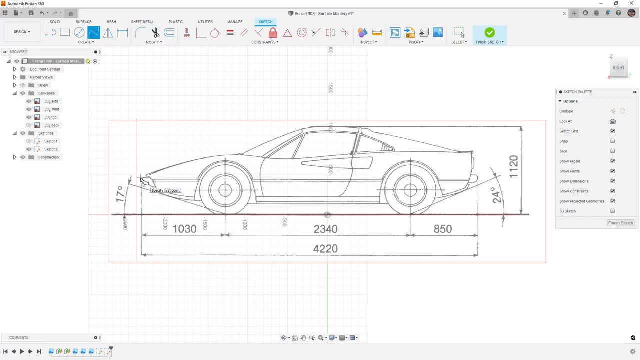 problem. So I'm going to hit escape to get off my spline tool and I'm going to hit escape to get Whenever I'm planning out surfaces. I am going to stop anywhere that the curvature changes direction. So for this we're essentially looking at a big arc, but then it arcs back up and 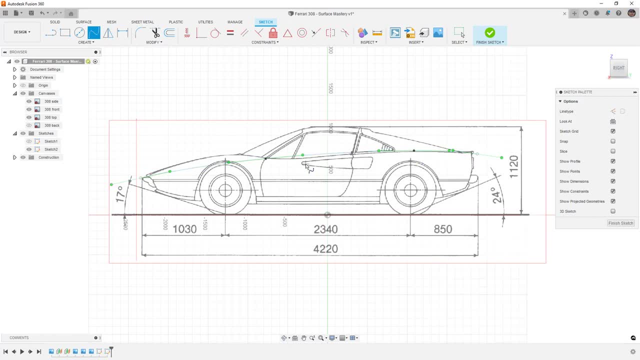 eventually it sort of dips back down at the back or levels out. This is a much harder spline for us to control and we generally don't want to use interior handles to control the spline because the curvature gets a bit messy. So if I start pulling this front edge here, you can see what's. 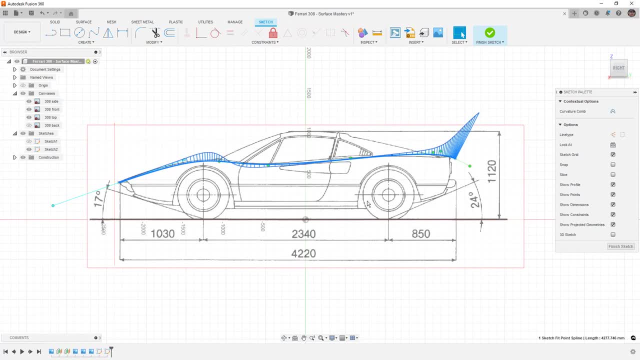 happening if I turn on curvature combs. We're starting to see this inflection point which we would expect to see right around the A-pillar or right around the sail window or the triangle window. We would expect to see it around here. So it means I might need to move this point around. 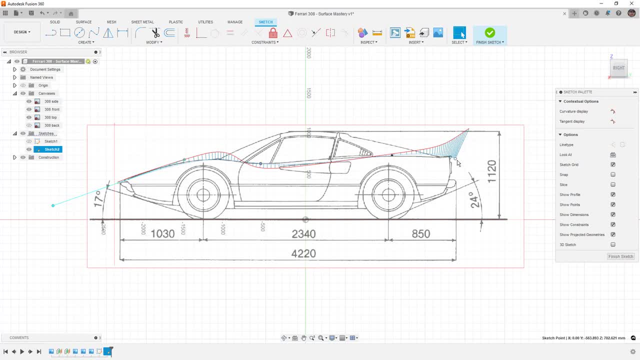 And then you can see at the back, we're seeing a rapid increase in the radius of curvature. but it's going the wrong direction. It actually needs this back curve here, actually needs to curve up, And what we end up having is again that inflection point. 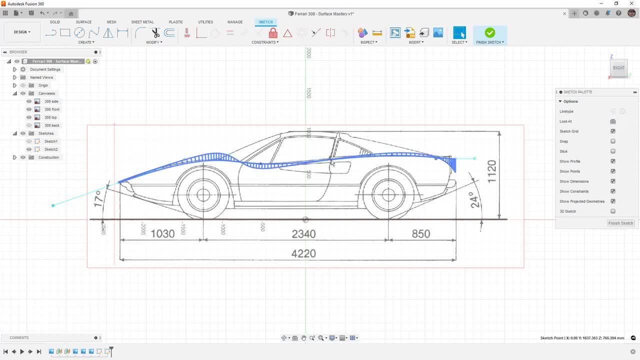 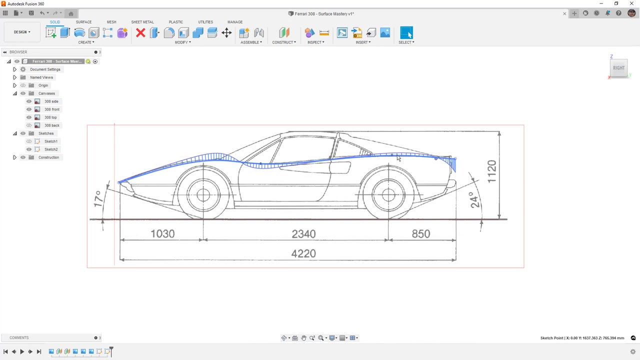 and we're having this center section here where we're sort of flattening out. We're going from convex to concave And that might be an okay result. The curve might be fine, but it's going to be less ideal because it's much harder for us to control that. 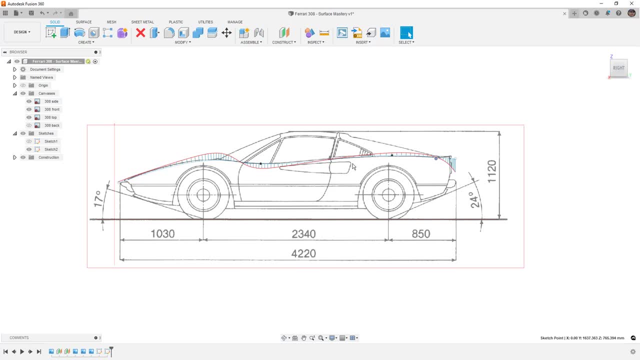 by using those handles on the end And it's not going to yield the same quality of results. We're going to have potential surface issues where we get spikes in those curvature areas. So ultimately, what I try to do is I try to build out my sketches so that I'm looking at a single direction of 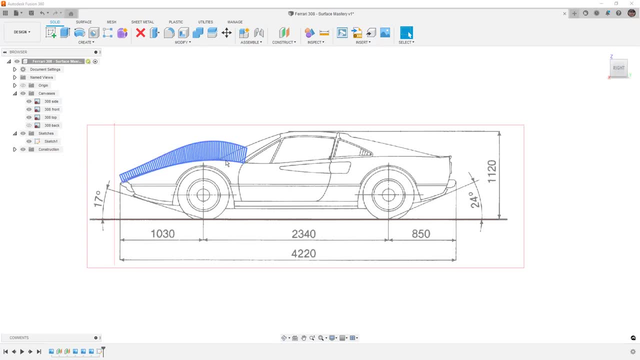 curvature. And, once again, what that means is, anytime we go from convex to concave, I'll likely determine that that's the inflection point where I start a new surface. Now, in this example, I'm actually stopping it a little bit short. I stopped it at the base of the A-pillar where, in reality, 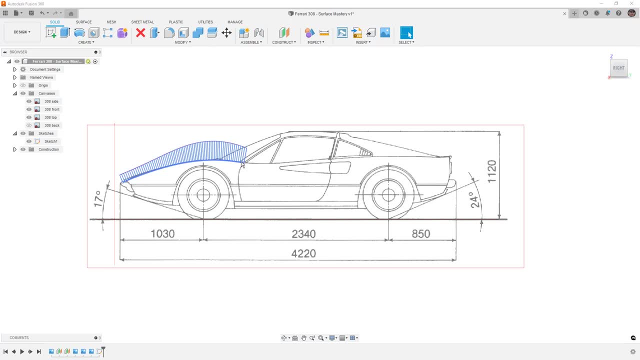 I would probably take it somewhere around here, So that way I'm not looking at another spline that's changing direction. It's oftentimes very easy for us to look at a blueprint and think, oh, I'm going to model the door I'm going to model. 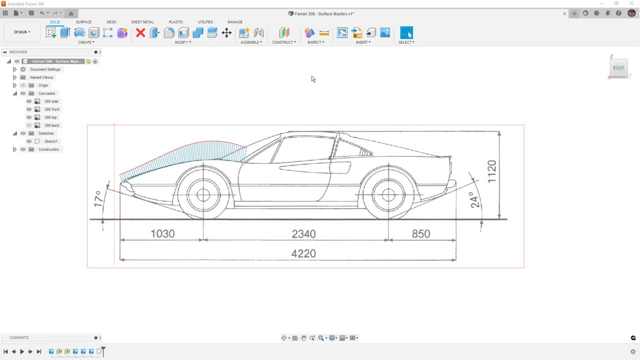 the front fender. I'm going to model the rear fender and model it in that approach. But you have to remember that these lines where they opened or they created the gaps for the door, those aren't necessarily changes in curvature. That just happens to be where the door opening is. 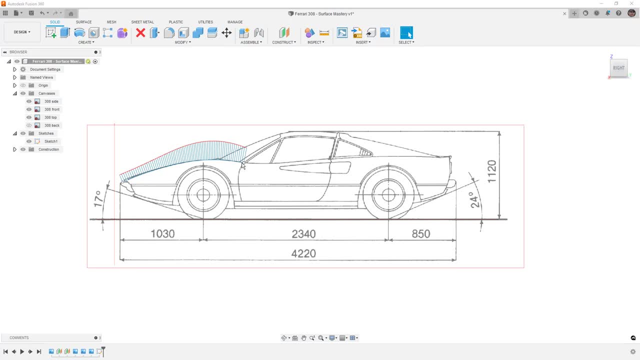 So it's important to try to think about the curvature or the shape rather than where the seams are. Now, there are some exceptions to that, For example, the bottom edge. here, this is going to be an exception. That's a hard line in the body And when we look at this from the top, 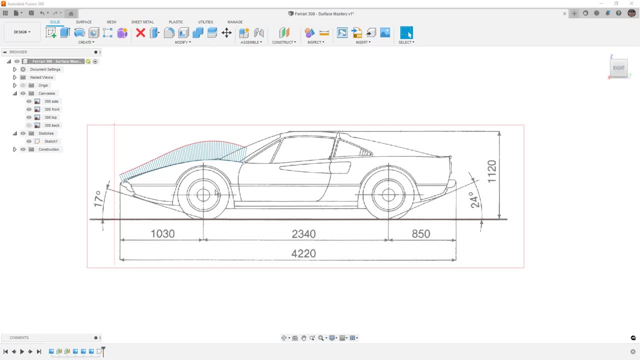 this is going to be the point in which the curvature starts to roll under. That's going to be really hard to model because we don't have a good view of what that looks like, at least in this set of blueprints. Now I do know that these cars, the shapes of them, do change and vary just slightly depending on the year. 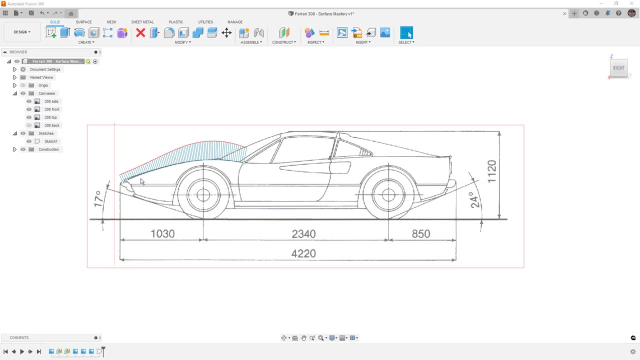 and, depending on various factors, Obviously there's aftermarket body, Liberty Walk and the wide body kit for these cars. There's tons of different directions that you could go with the body at this point, but all the ones that I've seen have maintained this upper fender line, So that upper fender line is a pretty key. 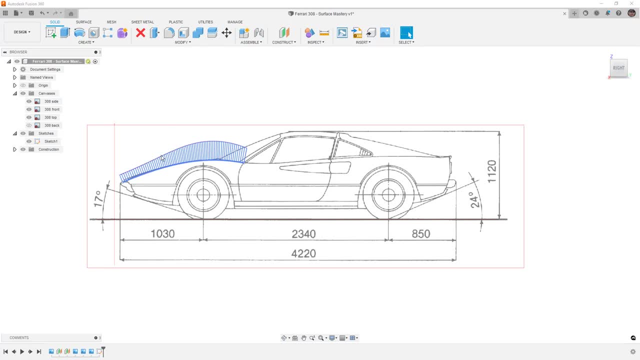 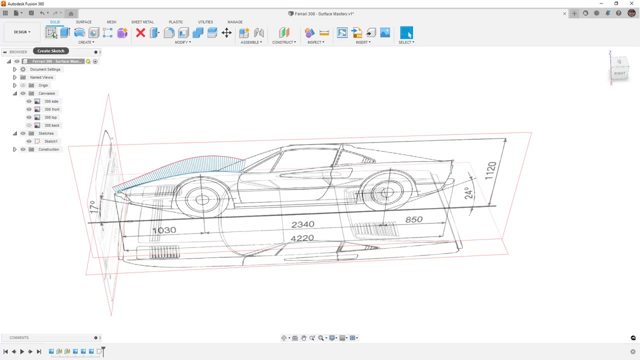 part of the design aesthetics here. So now let's talk about building out the 3D curve that represents this, And for that, what we're going to do is we're going to go to a top view and we're going to build out that same curve. I'm going to rotate my view so we can see a little bit. 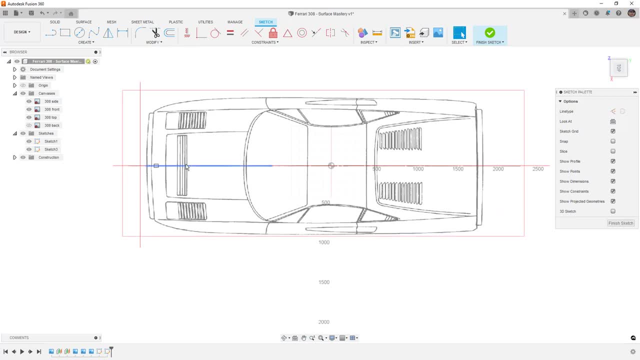 better Build out the same curve here. Now, one important thing I like to do is I like to project points, or the curve itself, by using P on the keyboard, And then I'm going to rotate this around, noting that it pushes it down to the base of the canvases, So you can see it down here. 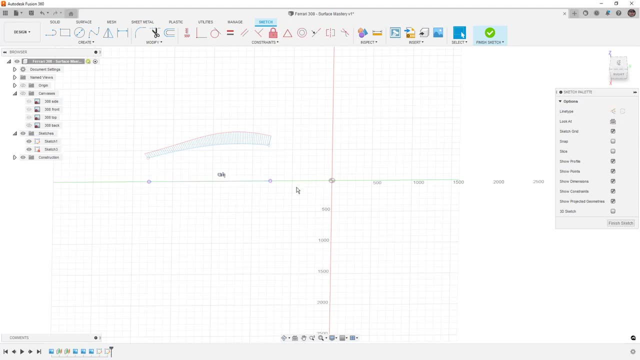 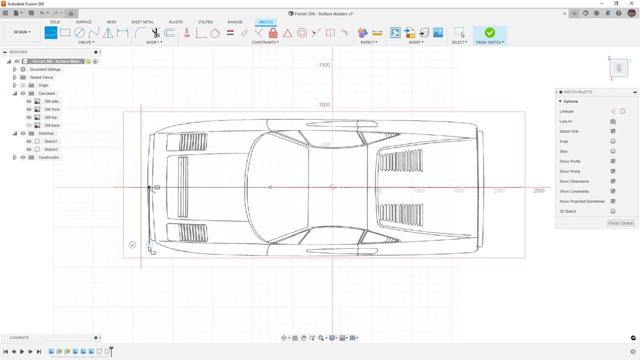 I'm going to convert it to construction because we don't actually need it And for the purposes of this video I'm going to draw some additional lines that aren't required, but they're just going to help us visually. So I'm going to draw a vertical line here at the front and a vertical 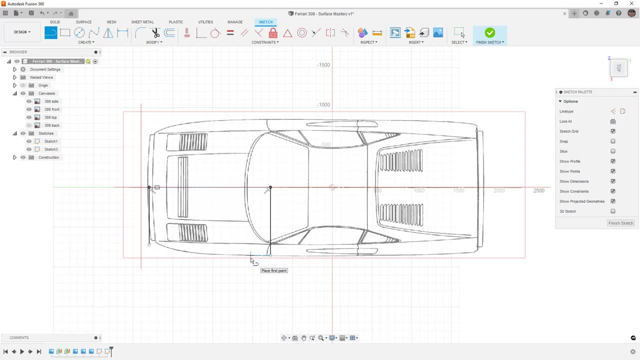 line at the back. The process here we need to think about when we're building curves in 3D is that if we're projecting 2D curves together, we want to know precisely where their end points are, And that's going to be important for us to build out the rest of the curve. So, once again, 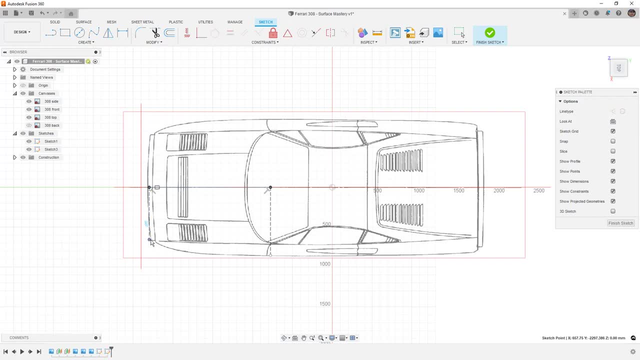 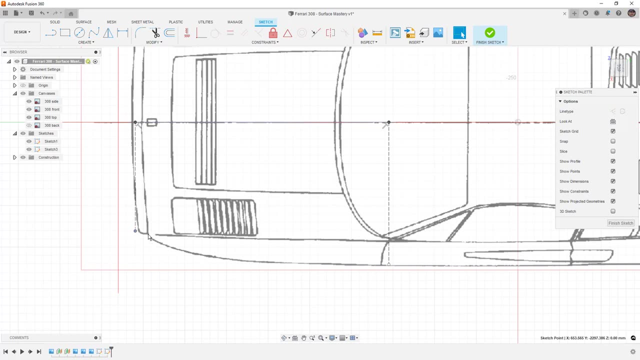 I'll make these construction and then I need to drag this down where I think that the fender curve would extend to, Because, remember, what we're doing is we're building this curve out. that's going to represent the upper portion of this fender. We did extend it slightly past in the 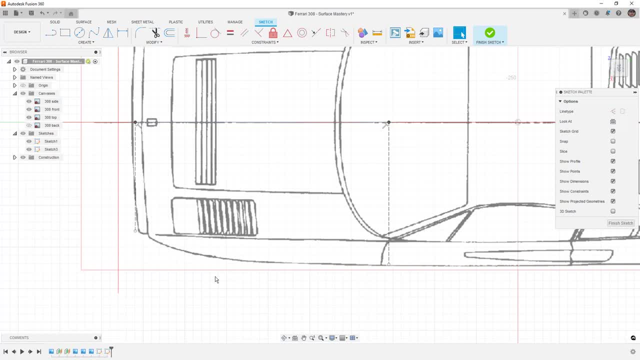 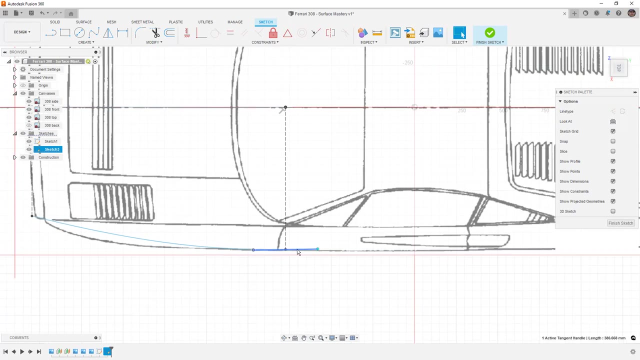 front so we can trim it back if needed. Now that we have these references, I'm going to use my spline to simply connect those two points: hit escape, and then I want to come back and create the curvature. Now the body here is going to be relatively flat, So I'm going to add a horizontal 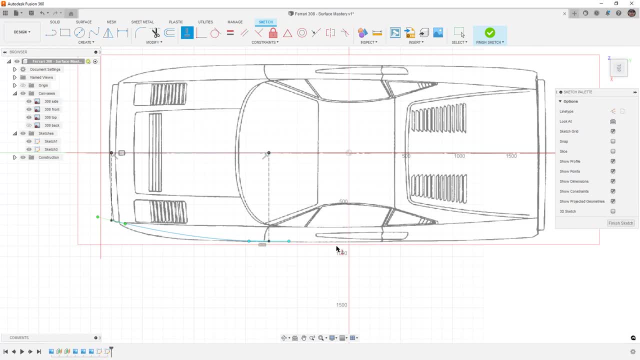 constraint and then it's going to start to taper back. at that point It'll flare back out for the rear fender a little bit, But for the most part, when you look down at cars from the top, they don't have nearly as much shape as you would think. Next, what I want to do is I want to change the 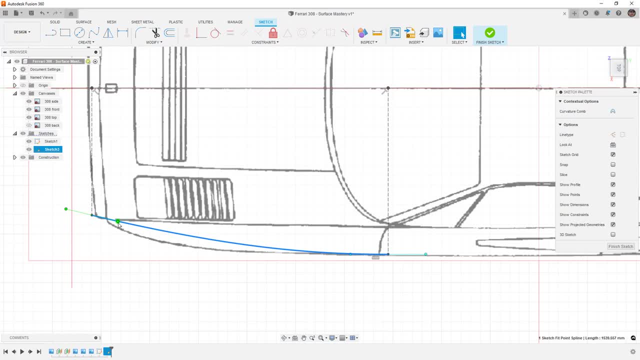 curvature so that it approximately matches the shape of the car. So I'm going to go ahead and change the curvature of the fender. Now. we have to keep in mind, too, that what we're doing is we're building out this line right here, And this is another common mistake. It can be very easy to 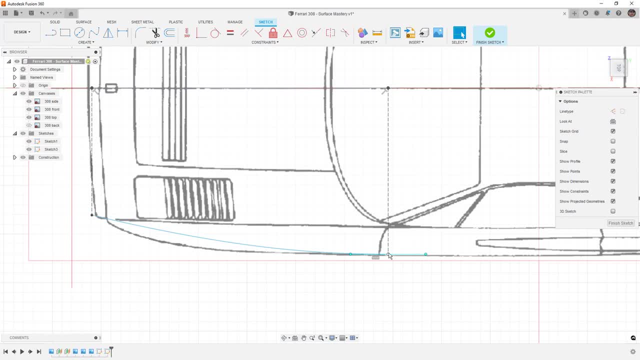 lose track of what you are trying to build. But with these reference lines it's very easy for us to just simply pull that line back up and maybe pull this line out a little bit. You can already see that we're relatively close to that shape. I want to do a quick check on the curvature combs. 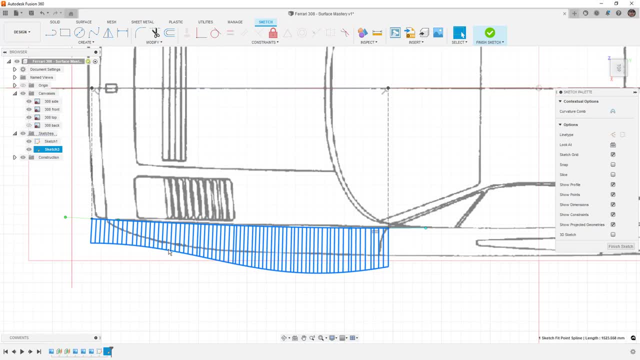 just to make sure that I'm not introducing a problem, and it looks like I am here. So what this is is that we are bulging out right in this area and then we're starting to go back out the wrong direction. Now this can be fixed by increasing the weight of the back handle or decreasing the 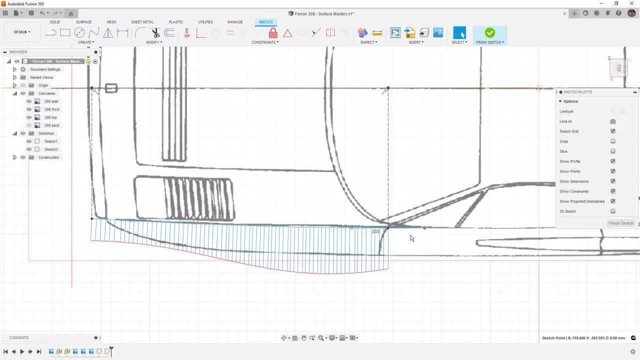 weight, depending on how your setup is. But what we want to look for is the length of this last curvature comb, which we can't really measure. We don't want it to be longer than ones before it. We want it to be shorter because we're tapering down at the nose of this Now. it can be pretty tricky. 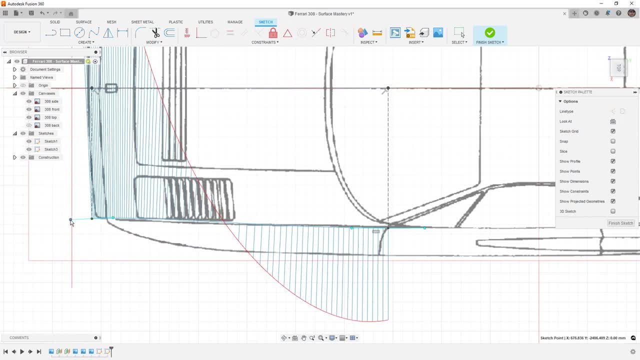 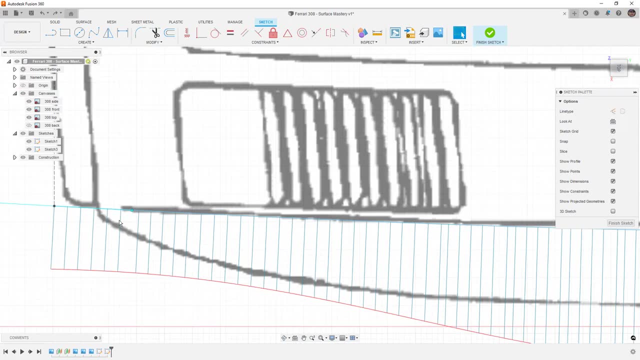 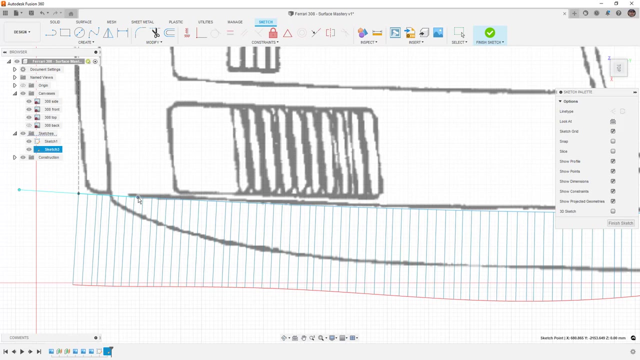 once we start to activate the second handle. See, it's very easy for us to sort of get out of shape, and it's almost impossible in this case. You can zoom in and get a little bit better resolution, but then you lose sort of the visibility of your curvature combs. So what we're going to do is we're just going to kind of play. 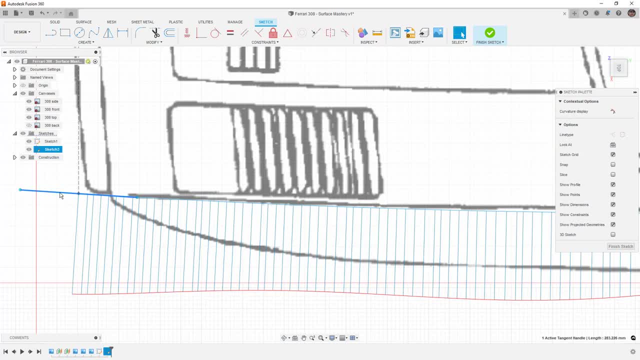 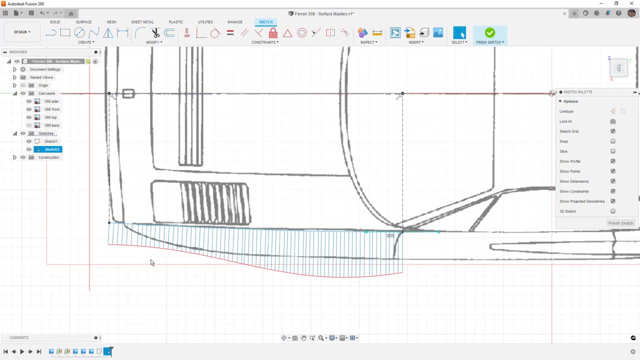 with it a little bit and at any point in time you can right click and you can deactivate the tangent handle and it'll go back to its original state. Now, the original state of a spline is going to be the least amount of tension in the spline. So if you activate a handle, especially at a midpoint, 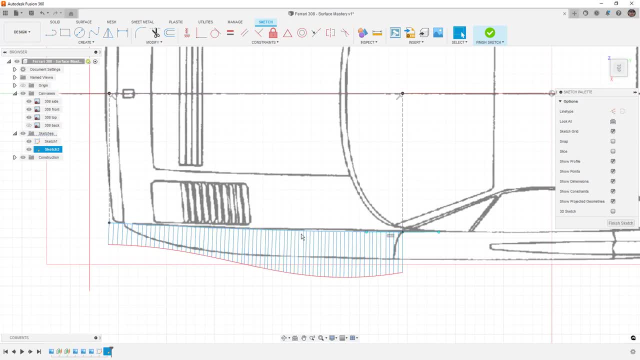 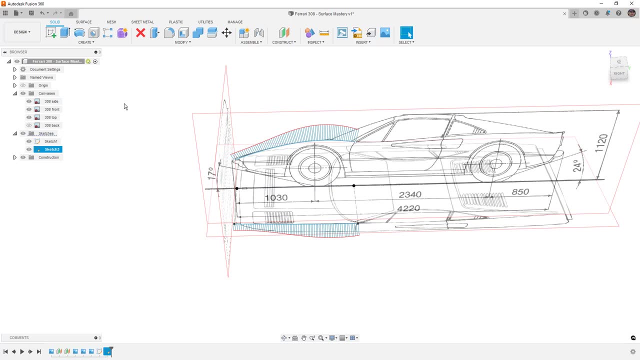 then you might need to select and deactivate those handles. I'm going to continue to run with it as is here, but just keep in mind that this does take a lot of playing around with. The next step in this process is for us to create a new sketch. It doesn't matter what plane We're just going to. 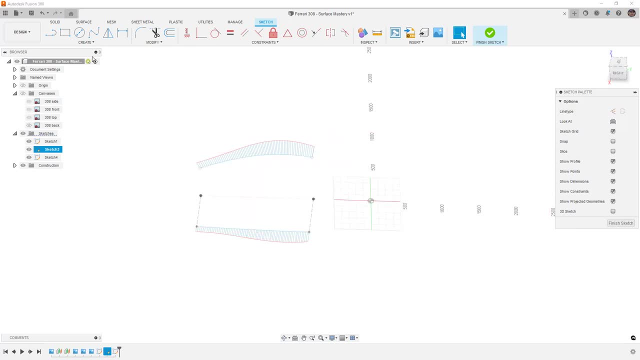 use the side plane for this example and I'm going to hide my canvases. Go to create project include and intersection curve. Now, the intersection curve is between a curve and a face or a plane, but we can also use it for two separate curves. We're going. 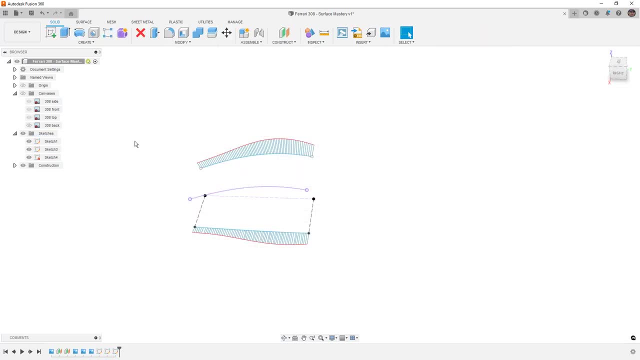 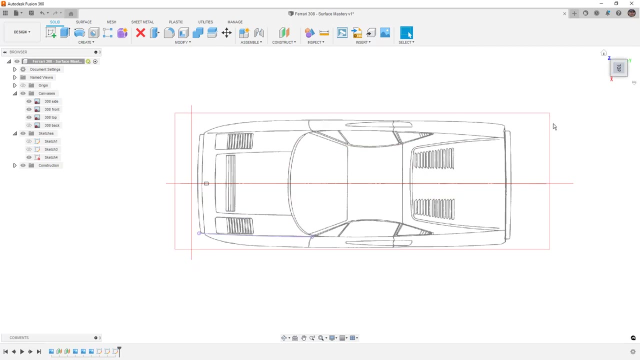 to project them together and finish our sketch. Now, if we hide sketch one and two and we bring back our canvas from the side, it should look just like the curve that we had from the side, From the top. it should look just like the curve from the top and from the front, where we didn't 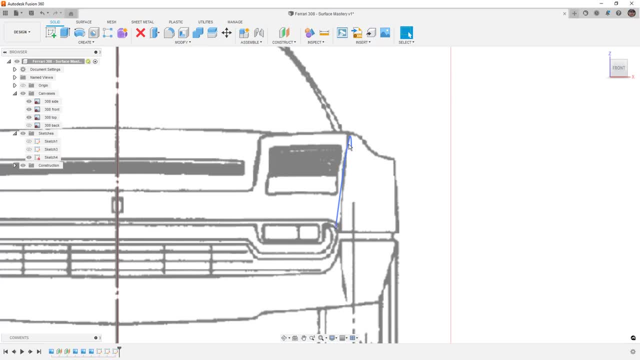 really have visibility of the entire fender, you can see that it's going up to the peak and then it's rolling back down. Now it is a little bit off here and it's partially based on things like the blueprint, the resolution, the position of them, the scale. There are all kinds. 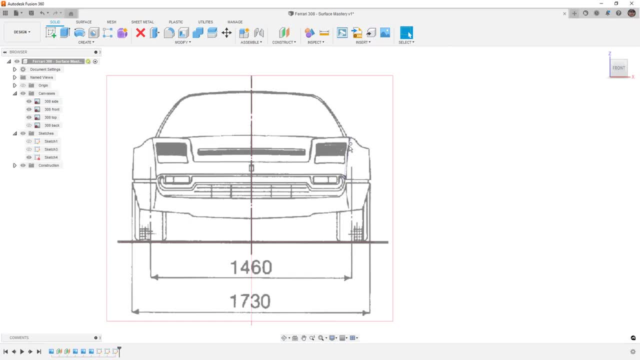 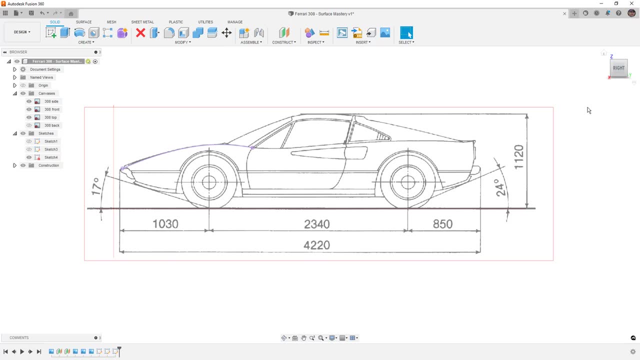 of things that can make it be off just a little bit, and generally we're not getting an exact replica of the geometry. That's nearly impossible to do. from images and references You're just going to get something that's visually close. That's basically the process of creating these. 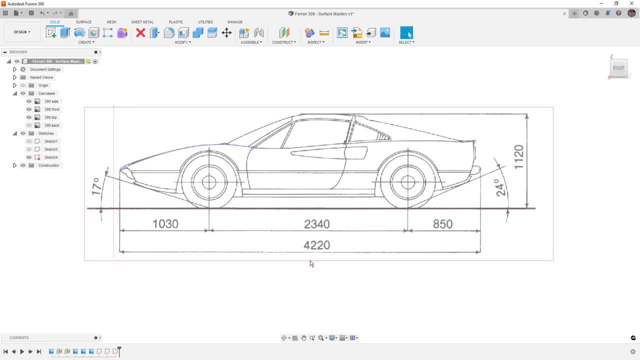 curves in 3D. There's a couple more things that we should consider, though. Now, if we're thinking about complex surfaces, the next thing to think about is how we want to model the rest of the geometry. Now, there are a couple of schools of thought here. 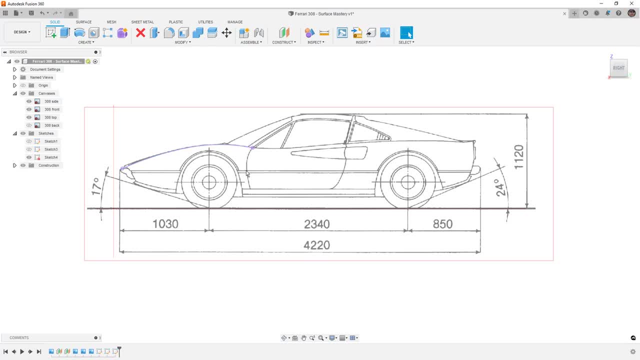 and generally, what I would do is I would build out the fender without the opening, without the arch, and then what I would do is I would come back and build that fender well and then connect them together, and the reason for that is because it's going to be very difficult with the surfacing. 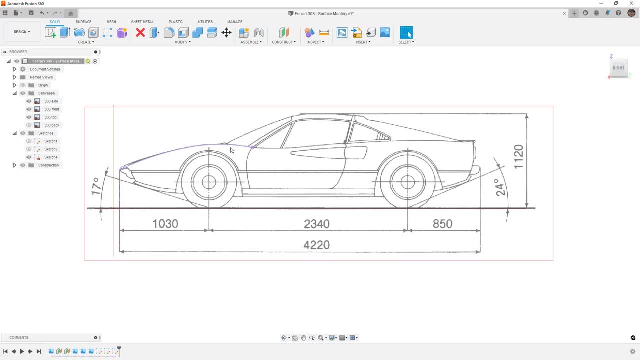 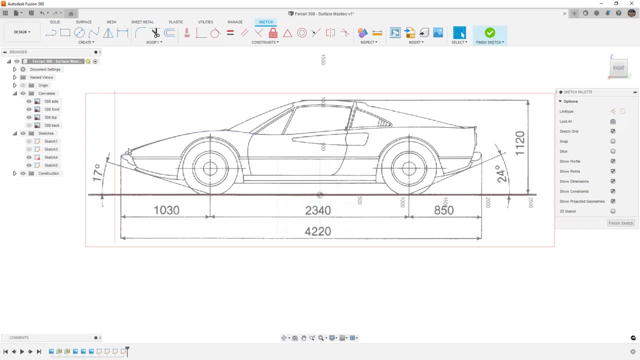 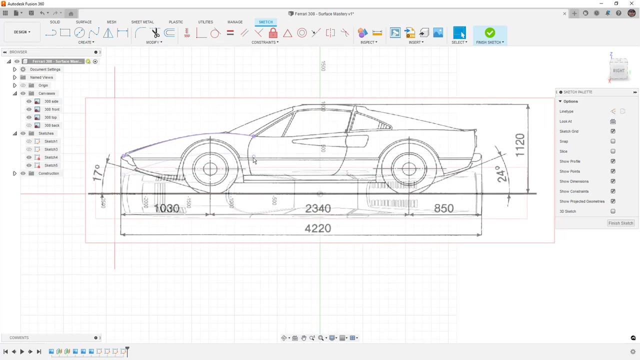 tools that we have and in most CAD software, to generate the shape that we would expect to see here in ARP CSB. So what I want to do is I'm going to create a sketch on the side. I am going to project this curve. Now, this is projecting the 3D curve, not any of the 2D curves, and I'm going 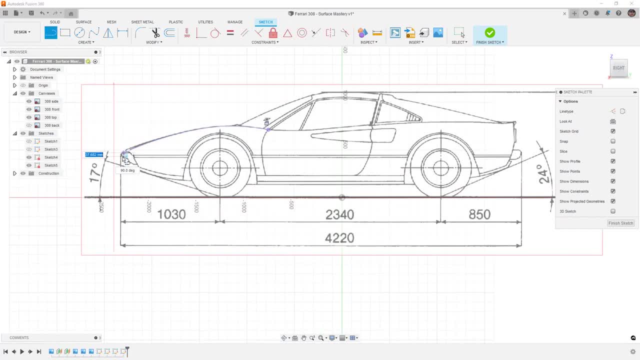 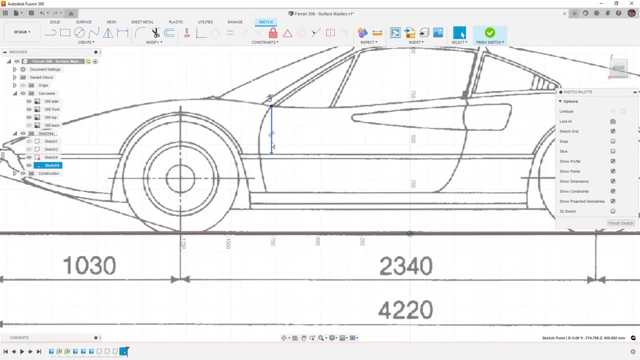 to turn it into construction and then, once again, just for the purposes of this video, I'm going to put some vertical reference lines in here. you don't need to have these here- you can use a vertical constraint- but I do think that it is important that we are aligning to some geometry. 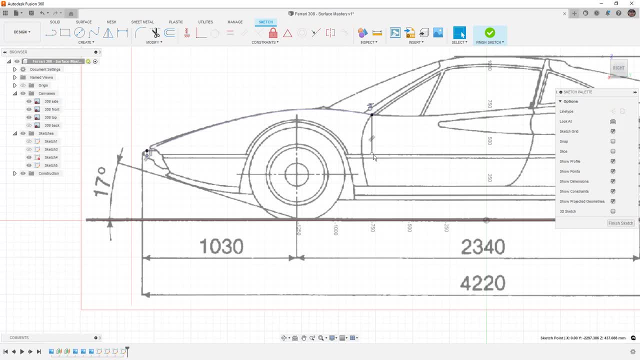 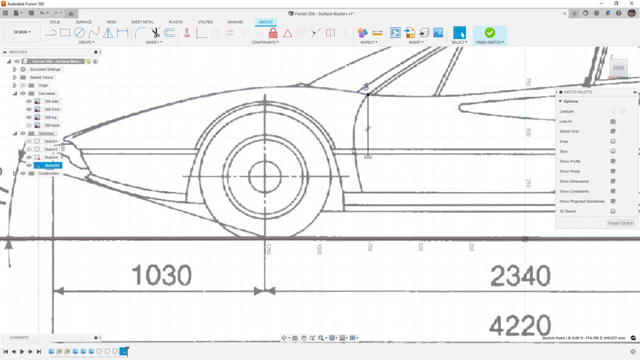 these end points. here the front curve is going to be really small, but I'm going to make their bottom points horizontal with each other and I'm going to over build this a little bit. I'm going to go past that first body line and I'm going to just come down to this second one here Now, just 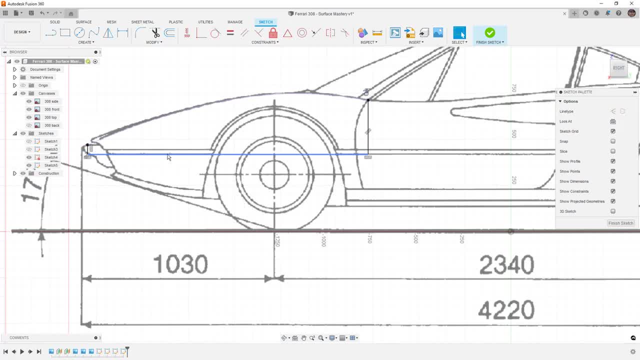 as a check, I'm going to draw a horizontal line here and make sure that it is hitting all of that geometry. Then I want to make sure that these vertical lines are construction, because we don't need them for the projection. Next thing I'm going to do is replicate that from the top, just like we. 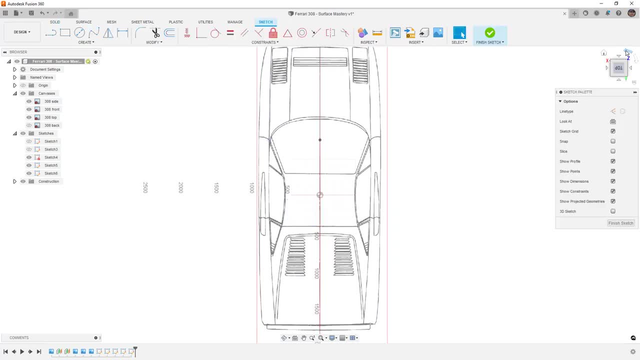 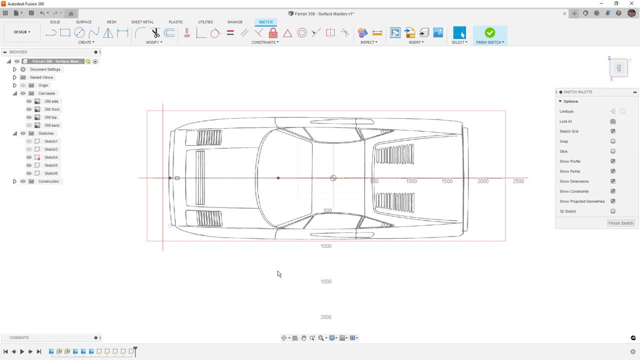 did before. Now you'll find that certain areas of cars will be very similar process. so when you're dealing with the fenders and the sides of the car, you're generally dealing with the side view and the top view. When you're dealing with things like the windscreen, you're generally dealing with the 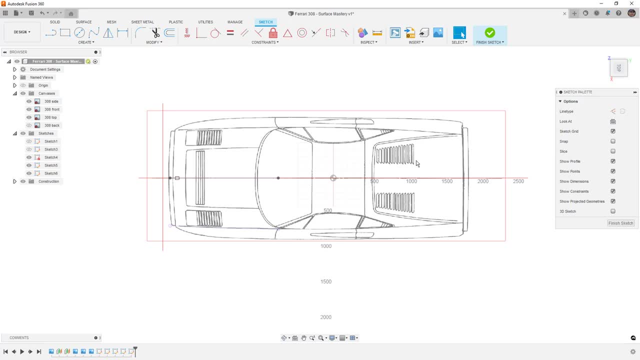 front and the top, and when you're dealing with the back of the car, you're dealing with the back and the top. generally There are differences depending on curvature, but that's just the general process of what you get Now from here we have this straight line. 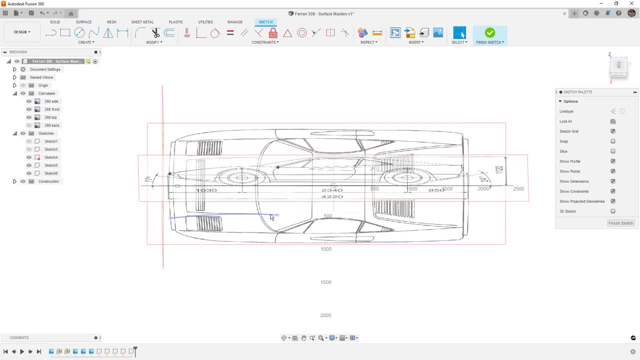 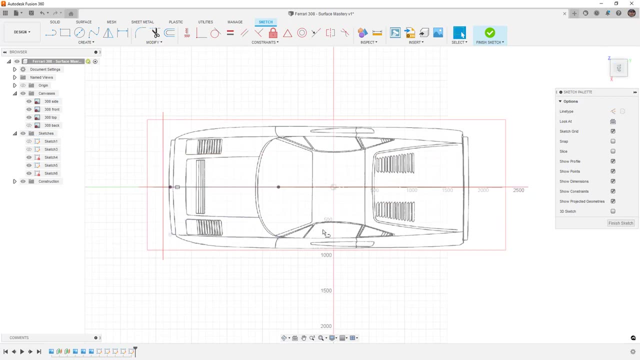 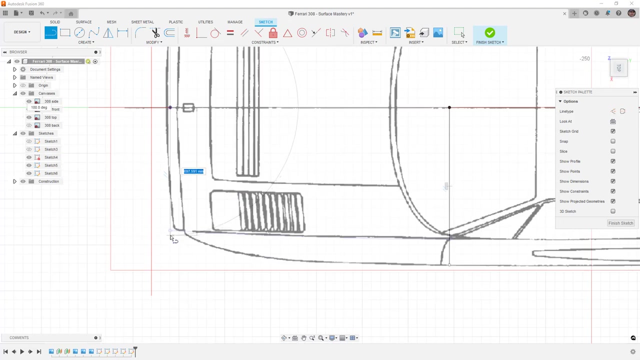 we have the end points on that projection and we have the points here. We could project any of those, but I'm going to just take the end points and use p to project those and once again just add those straight lines Again. the main reason I'm doing this is for visual reference for the video and 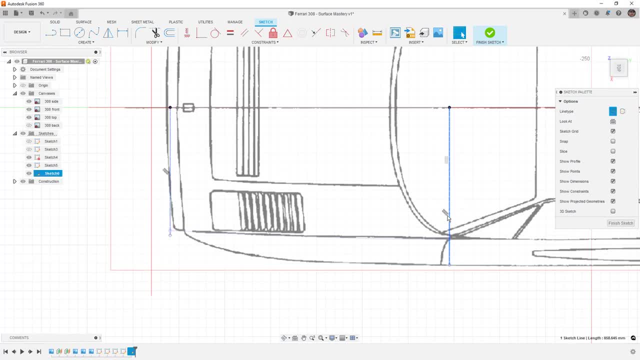 it's not needed when you're doing this in on your own. if you're just trying to create 3d curves, A vertical constraint works the same, but visually this helps, especially since these are hard to see through blueprints. Then I'm going to take the end points on that projection and we have the end points. 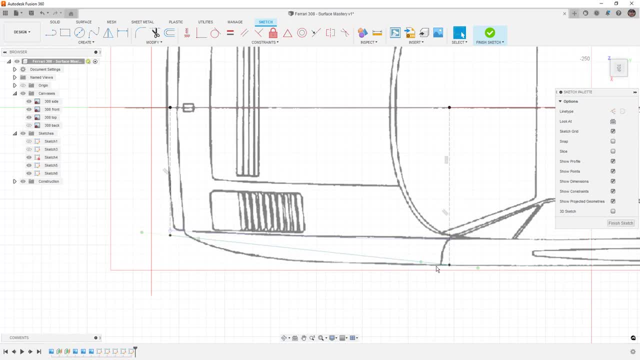 here. I'm going to start to connect those points. I want to minimize the curvature influence I have, so horizontal here, and I'm going to start to pull this out. We're not going to perfectly match the shape, and the intent here is not for us to fully model this car. anyways, You have to spend. 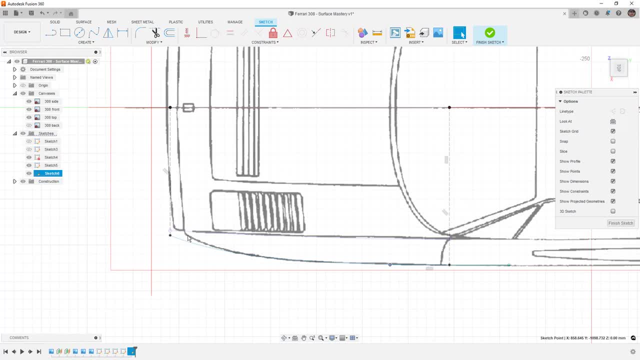 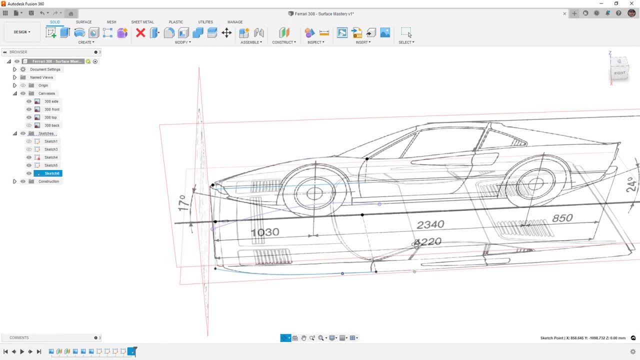 a lot of time planning these curves out, looking at reference images, and it's just not the intent of this video. We're going to approximate the shape again. we can always trim it back and build out this corner later as well. well, so you'll notice that i didn't turn on curvature combs here. i'm fairly confident in 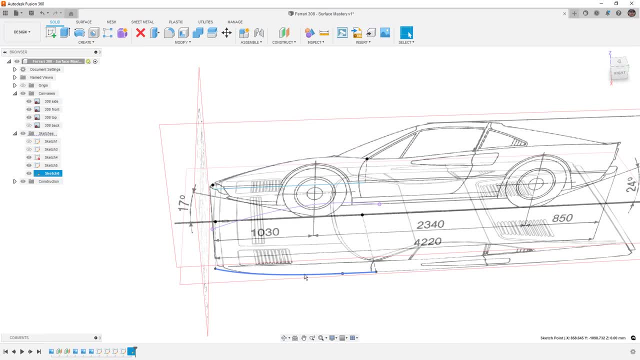 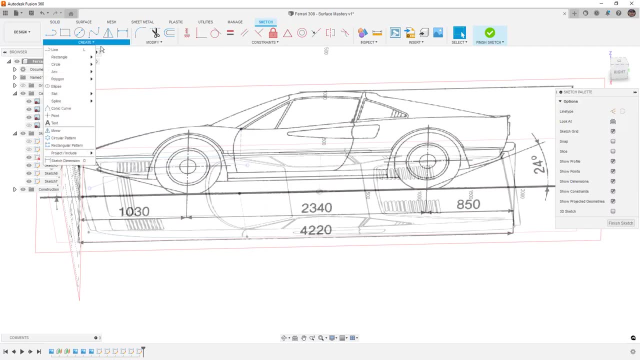 the shape, because i only modified one handle. if you want to turn those on and play with them, by all means go ahead. then once again, we're going to create another curve on the side. we are going to do project include, intersection. take the straight line there, the top down, and say okay, and then 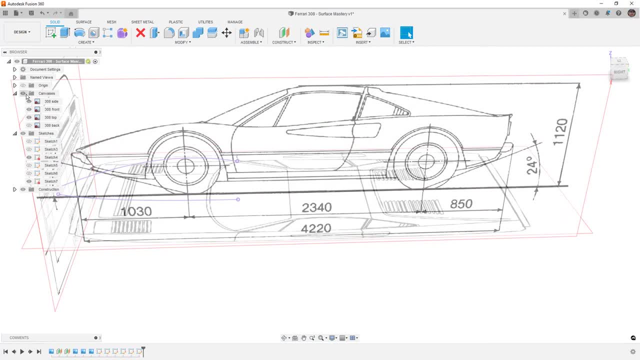 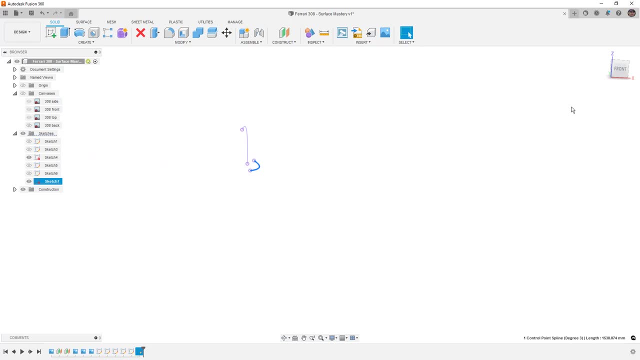 we'll hide the two previous curves that we use for the projection. now, if we hide the canvas, we now have the upper edge of the fender and then we've got the one that goes through the wheel. well, so when we look at it from the front, this is essentially the shape that we're looking at. 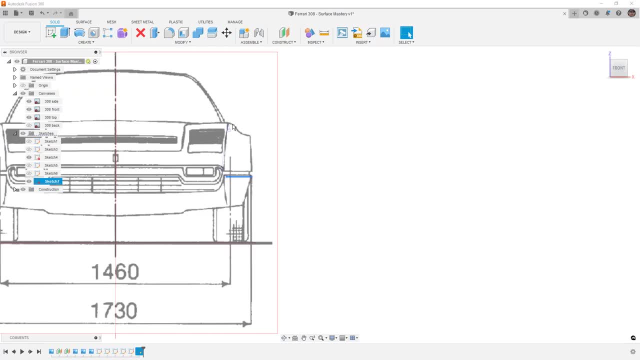 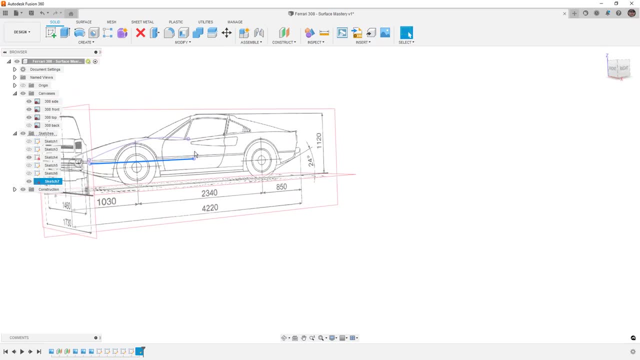 however, we need to tell it what's happening between here and again. various years of these cars are going to look a little bit different, but what we're going to do is we're going to build out the curves at the back, at the front and in the middle. now, that's not necessarily required. 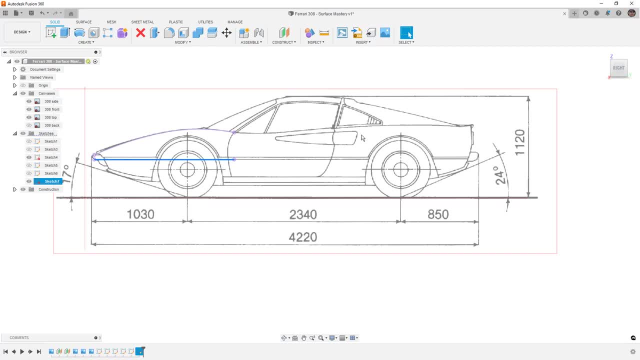 so, for example, if i was doing just the middle section of the car, the consistent see of the curvature there means that i probably don't need to fully build out these guide curves. but for our purposes, because there is such a drastic change in curvature around the fender- 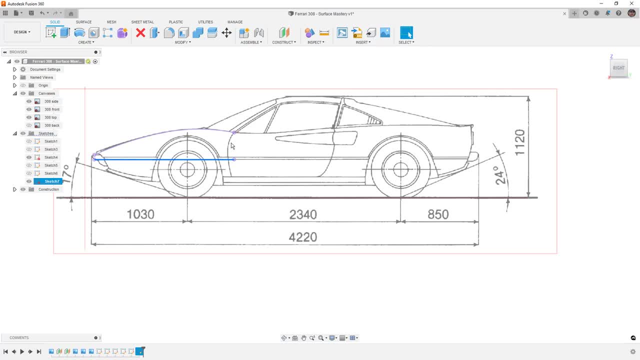 around the wheel, i should say, and then at the front and the back. i think it's important that we understand how to build out these curves. so what i'm going to do is i'm going to start by creating a sketch and we have to think about the geometry, how we're going to project this. 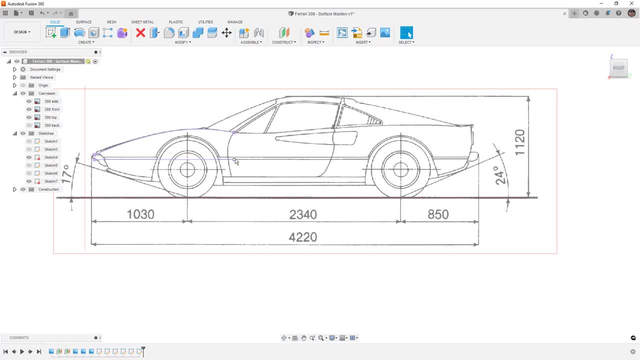 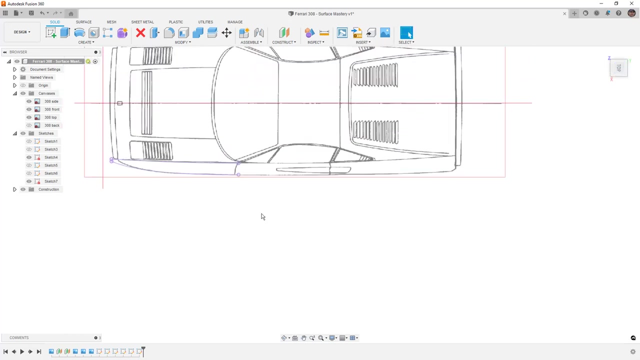 now everything we've done so far, the starting point and the end i can take, and if i start here and i get this much better, so within my an angle piece of paper right again goes our square, simply. so i think that this is looking very beautiful, all right. 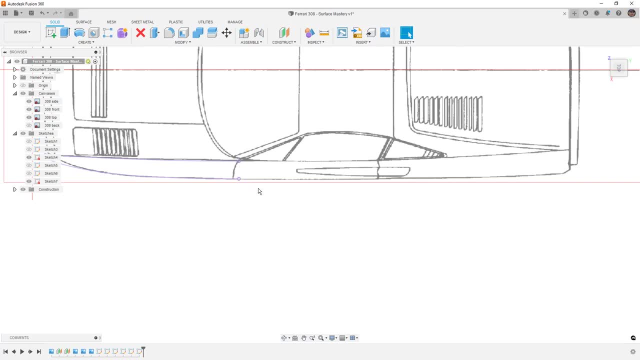 so what am i going to do? and i'm going to just set this water at the top. i want you to just 세계 fix that to make sure it's thinking it bishoe, appeasing the bottom, and once that's accepted, it's going to get nice. 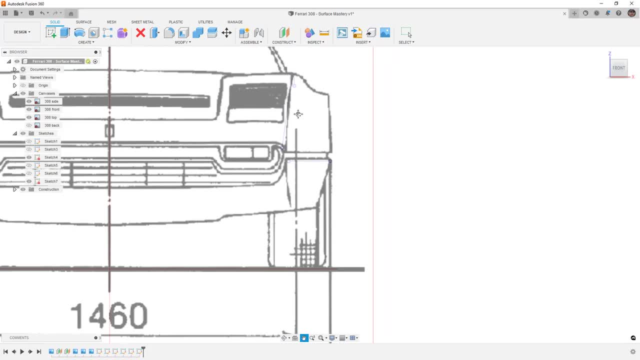 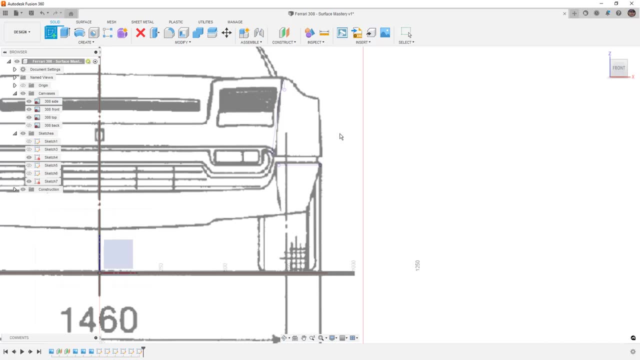 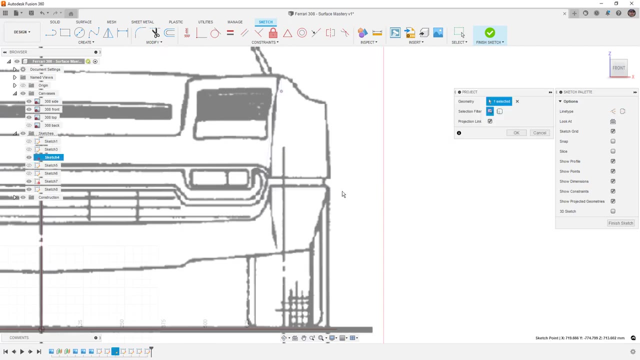 kind of glass, a straight up. so again, here is where we really need to start to think about the shape and we have to make some design decisions. So I'm going to start my sketch from the front, knowing that from the top or the side it's just going to be a straight line, and then P on the keyboard, we're going to project just the. 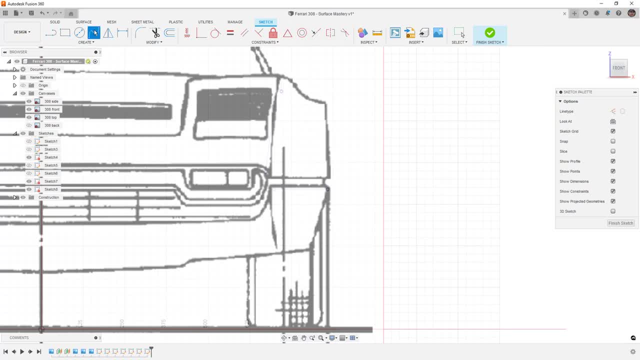 end points. The end points are all we really need to hit, and then we're going to create a spline that goes between them. So at this point we have to think about what we would expect the door to look like on this car, based on where our handle is going to be. So I would imagine that at this 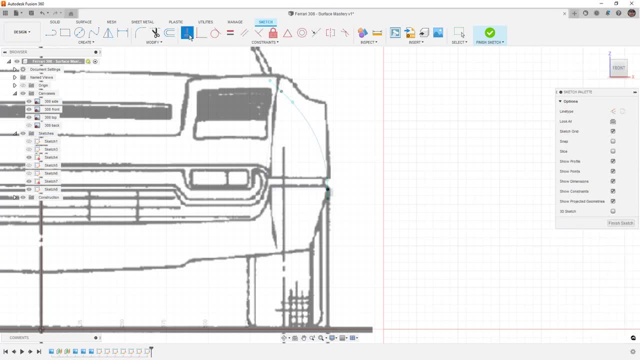 point that we're going to assume that this line is vertical and that's because the curvature is going to start to roll under here. and that means, as we build out the curve below the door or below this midline, then we know that the tangency is going to be vertical. at that point, at least at 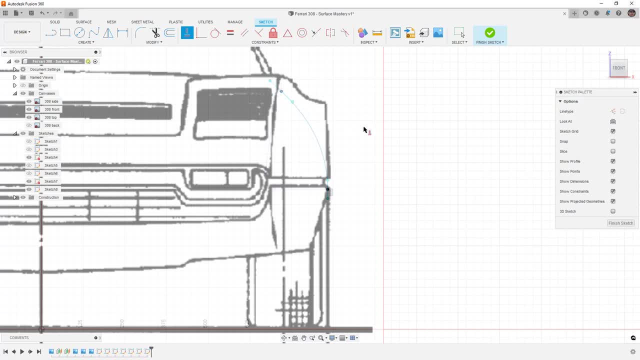 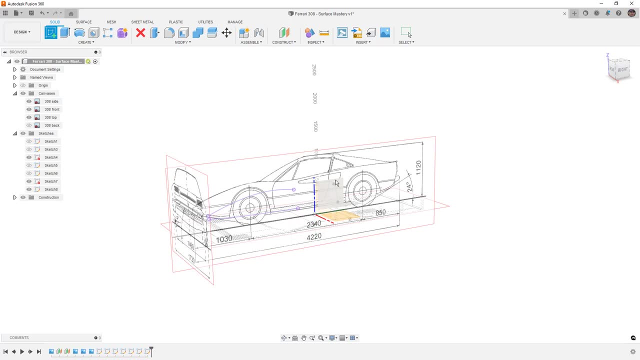 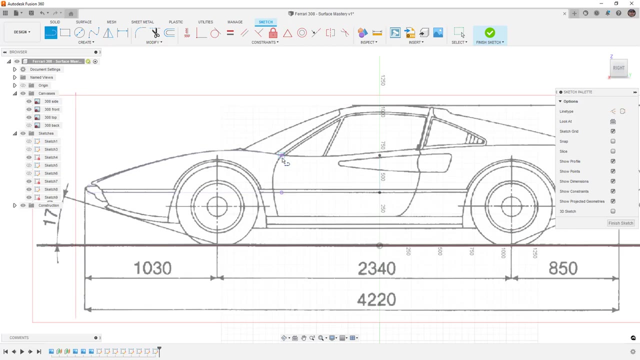 this edge And then I'm going to roughly approximate what I think that the shape looks like. Then, when we go to our side view, let's go ahead and create a new sketch. We're going to do the same thing- P on the keyboard and project these two points, and then all we need to do- because we created them- vertical. 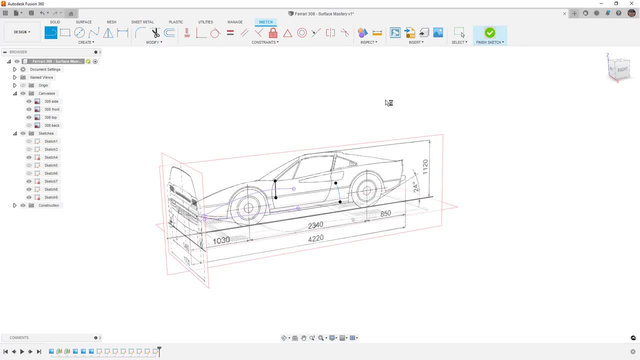 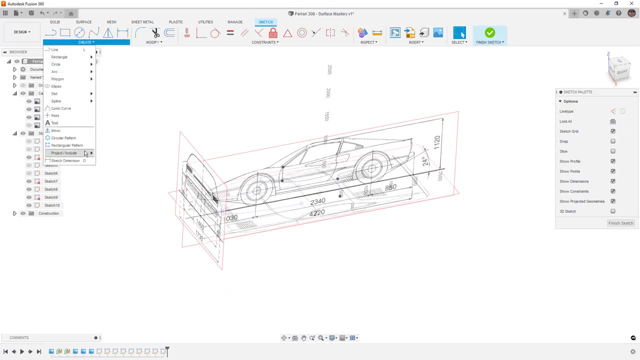 relative to each other is just create a vertical line. Now, once more, we can create a third sketch. doesn't matter what plane it is, because all we're using this is to contain the projection. So we're going to do an intersection curve to project these two out until they intersect, and then we can hide. 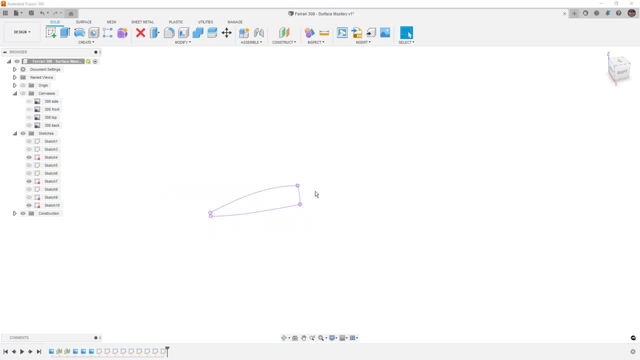 those two. So what we should have built is a curve that exactly touches those points. Now, the reason this is important is because when we go to do something like a surface loft, it's going to be really picky about that curve being a guide. It's going to have to touch everything. So, making sure that we take 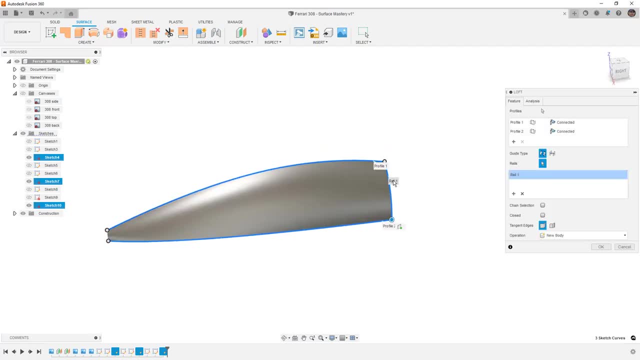 the time to add those constraints and build it out is going to be important. Now, what we could do is we could leave this as is, but the front is sort of just doing its own thing. We haven't defined anything on the front yet. If we want to define what happens at the front, we need to once again create a sketch on the front. 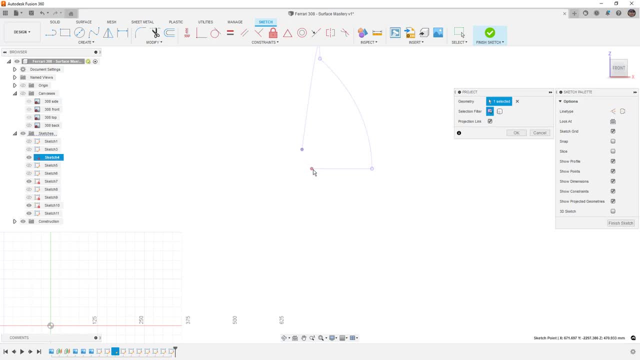 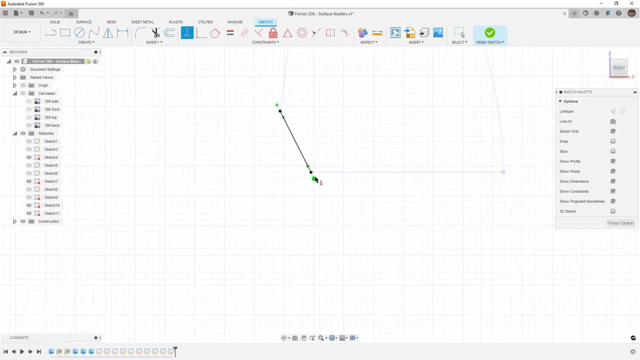 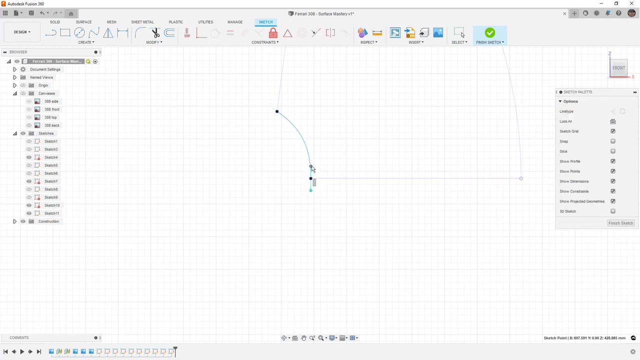 P on the keyboard to project these two points. and then we want to build out our spline- and once again I'm going to assume that this handle here is going to be vertical- and then I want to manipulate the geometry. and we can do this either with just the handle that we added a vertical constraint to, or 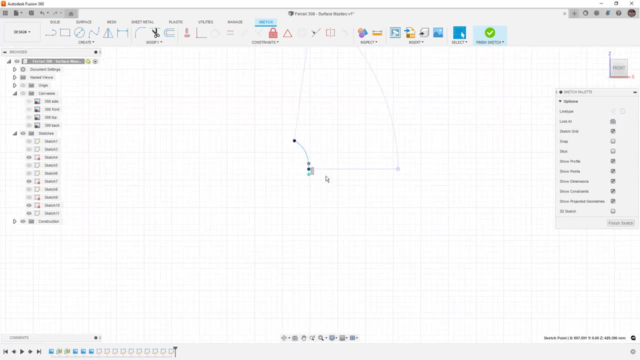 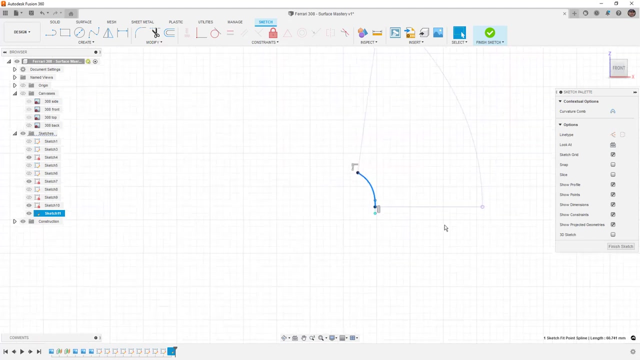 we can activate the upper handle, but remember, the less control that you have, or at least the lower control tangency handles that you activate, the better your overall geometry is going to be. So the curvature comb is going to be much smoother if I don't enable that upper handle. So that's. 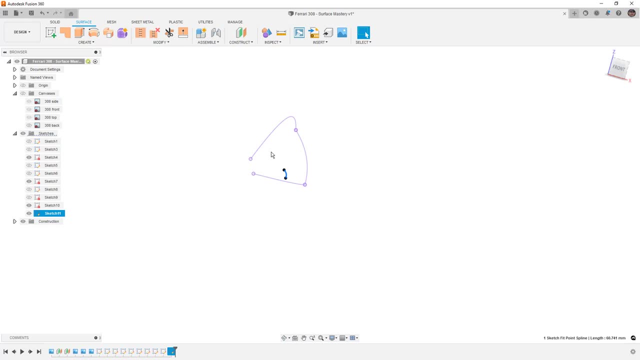 always what I strive for whenever possible. It's not always possible, but sometimes you can make it happen. Then for that front edge, once again, we'll do the same thing. P on the keyboard project. these two points make a vertical line. Another thing that you could consider when doing this is: anywhere. 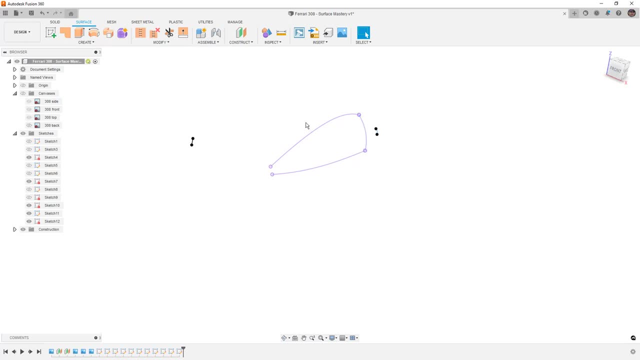 you're building out your geometry, you can create a plane, and creating a plane will allow you to avoid making these extra straight handles. Now, it's not always, again, it's not always possible, but in some cases, building those planes out at the points where you're going to divide up the body of whatever. 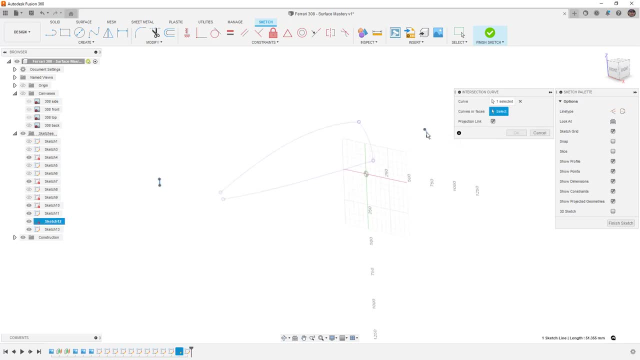 you're designing can be a helpful process. So again, we're going to create those. now we should have a curve in 3D that attaches those points. I can hide the two previous curves and you can see it's got some even more interesting changes, So it's always a good idea to rename these. So I'm going. 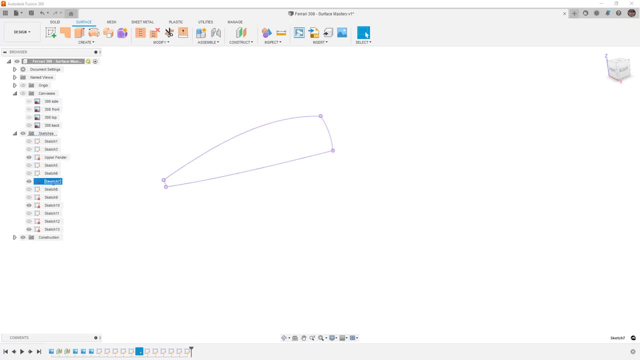 to call this upper fender, and this is going to be my mid fender, and this one is rear and this one is front. Now, obviously, if I was modeling the entire car, we would have hundreds of sketches, but we're only just doing this portion of the fender, so we're not really too worried about it. 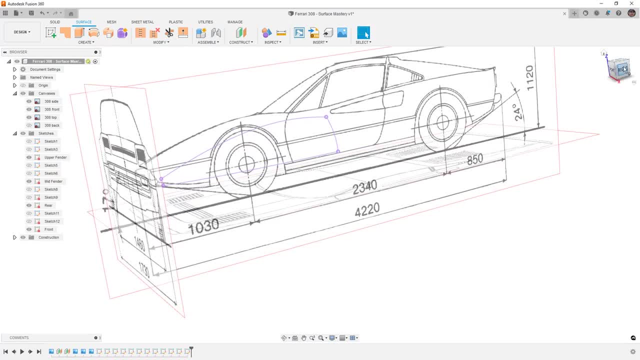 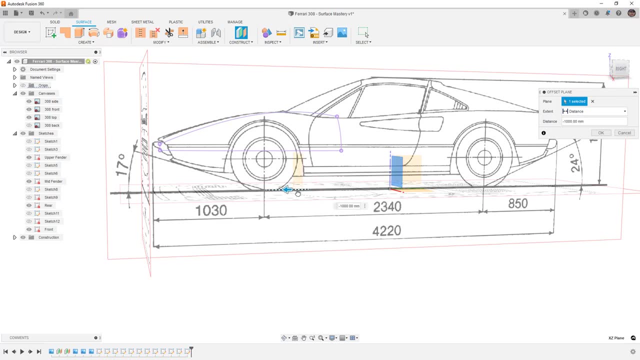 The next thing that I want to do is I want to bring back the canvases and I want to build one more guide curve and to do this, I'm going to create an offset plane. I'm going to go ahead and view this from the side and I want to put it roughly in the middle of the wheel, so I might. 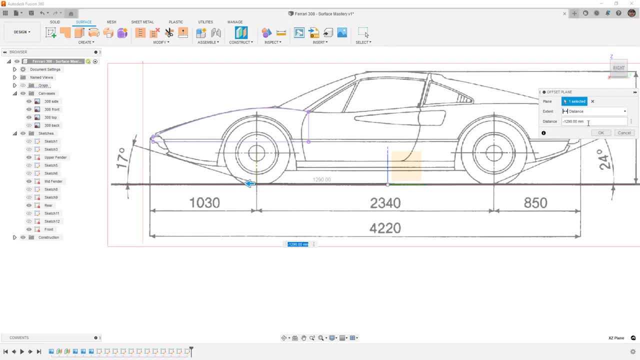 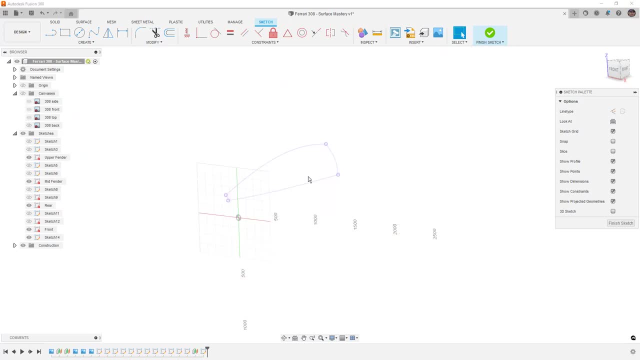 need to zoom in to get the resolution that's close enough. and now I have a plane that I can sketch on. and what I want to do now- and I'm going to go ahead and hide the canvases because I'm just going to approximate the shape- is: I want to go to project, include and intersect. I want to find the 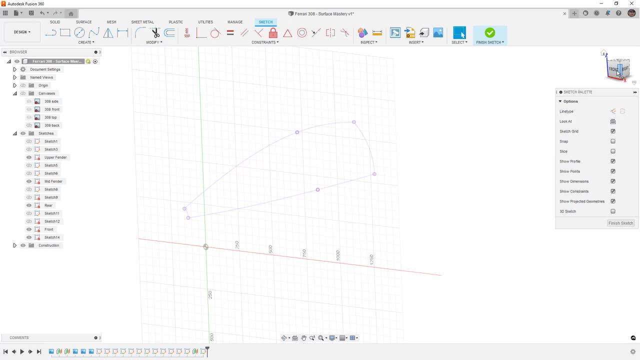 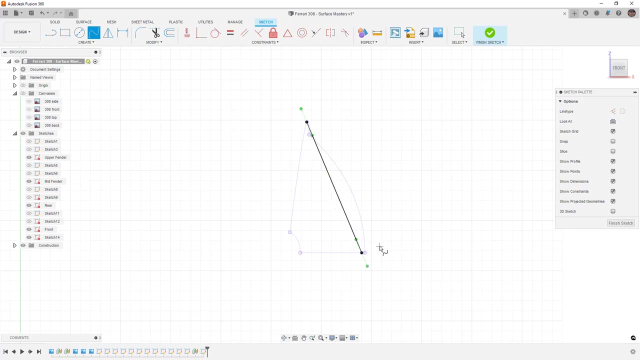 points where that plane intersects my spine, and the reason for that is because we need to attach to it, we need to know exactly where it is. so we're going to go to those two points once again. we're going to give a vertical constraint to that handle and then we're going to start to manipulate the. 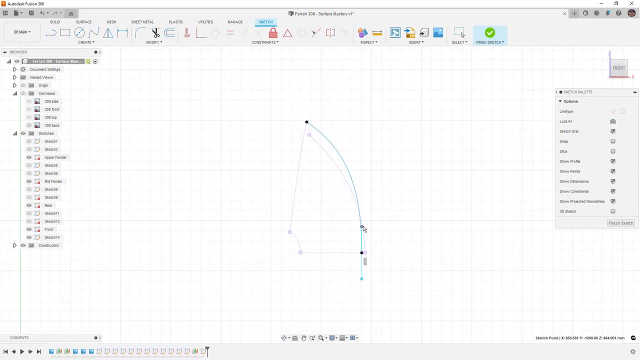 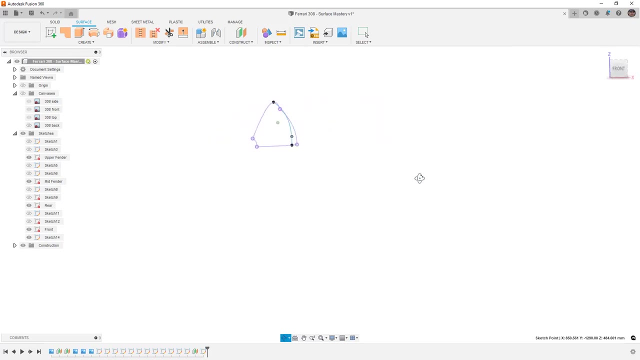 shape now. remember that at this point the fender is likely going to bulge out a bit more because we have the wheel well, so we're going to have to just once again approximate. but now we don't need to project anything into 3d, because we created a plane exactly where we want it to be, and we're 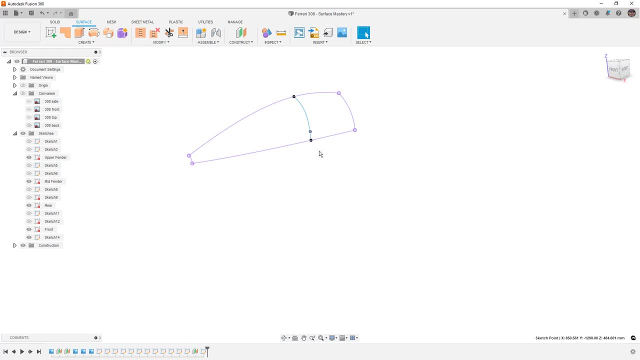 going to get the shape. that's exactly where that curve needs to be and we just attached it to our spline. now you could build out more curves if you wanted to really drive the shape of this, but in this case we need to take a look at lofting and we can either go from these small sections using the 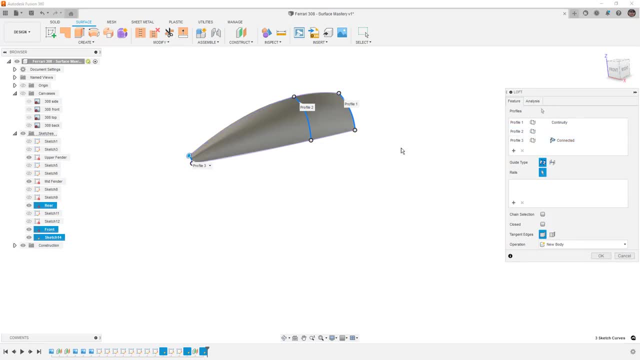 upper and lower edges as guides, or we could go from the upper and lower edges and these could be the, the lofting profiles, and then the rails, or the three profiles would be the, our guides, the rails that go in the middle of it. so that gives us the general shape that we're. 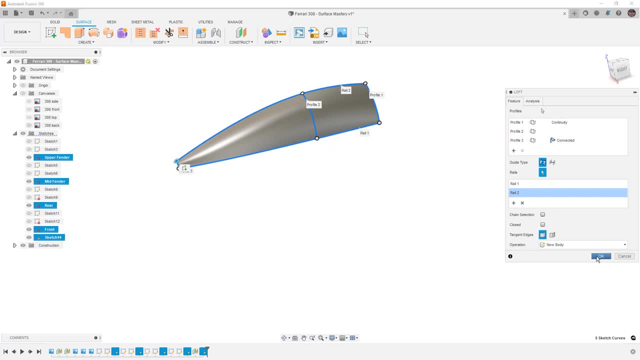 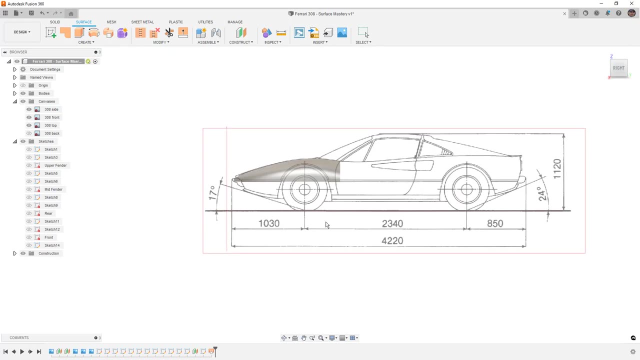 looking for it looks pretty good. we could probably do a little bit of work up front, but that gives us the general shape of the fender. if we bring back the canvas, we look at this thing from the right. essentially, what we did was we built that upper portion. we look at it from the 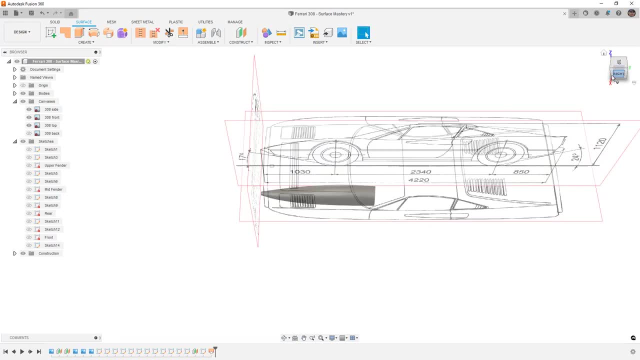 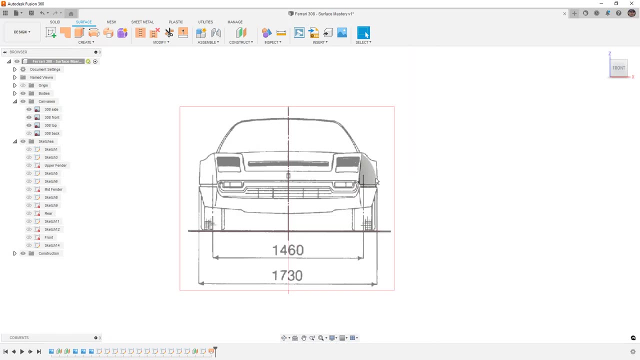 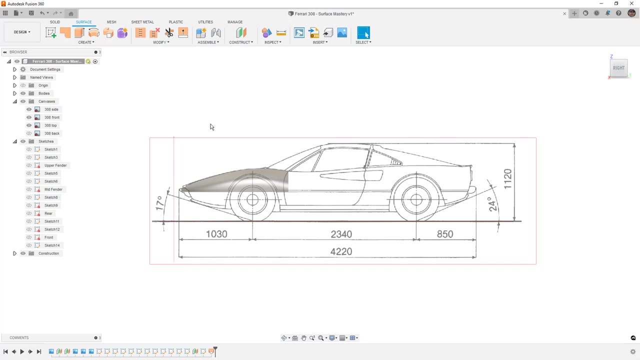 top, it should match the shape. if we look at it from the front, it should approximate the shape without the flare for the wheel. well, so that's again that's going to be the general process of building out those curves in 3d. there's obviously a lot of nuances to this and it's very situational. 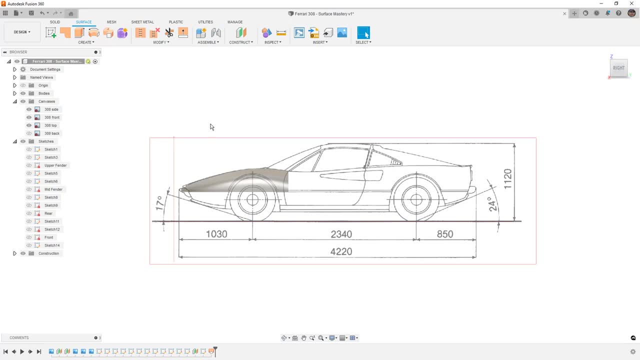 it's very dependent on what you're modeling. but if you're trying to model a car, then the way that you go about it is just like we did: you build out your 2d sketches, you project them into 3d to build out those main defining lines for your curves. and once you have those main defining, 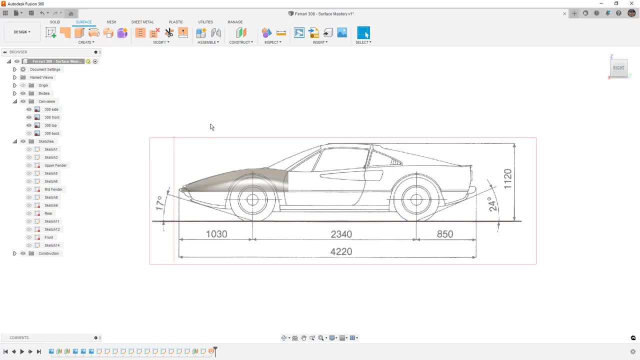 lines, you go back and you build 3d sketches, you build out those main defining lines for your curves and once you have those different guides or rails to help control the geometry, now the difference between doing it from scratch like this and then building to the next level, let's say the bottom of the fender.